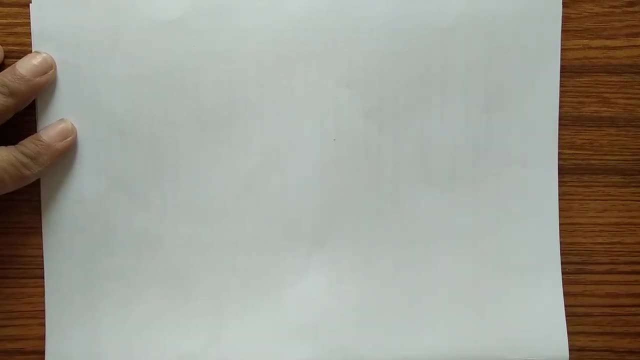 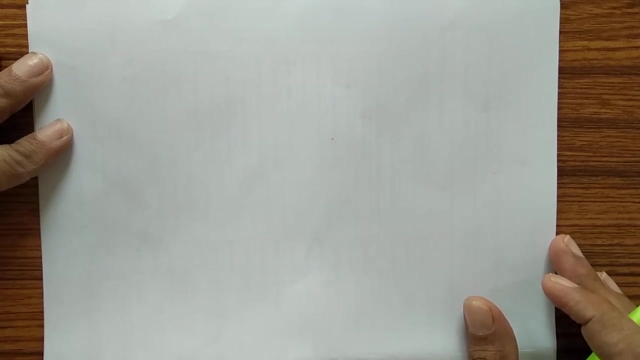 Welcome to our channel Concept in Mechanical Engineering. Here we will study the entire syllabus of mechanical engineering, which will be helpful for your semester examination, gate examination, IS examination and other competition examination. First we will start with the most important and interesting subject of mechanical engineering, which is thermodynamics. 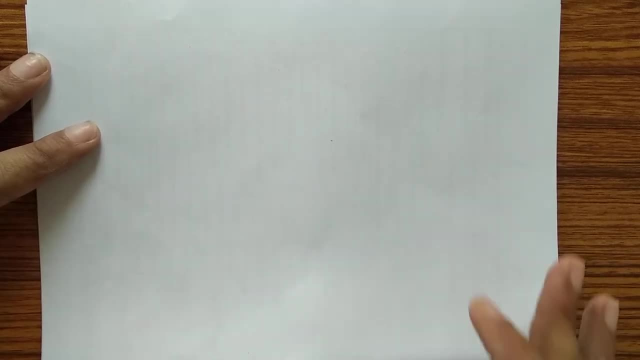 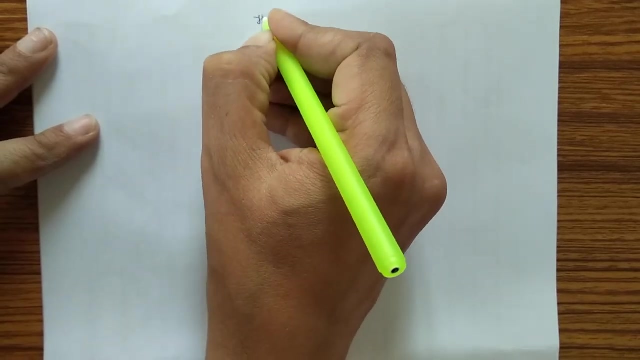 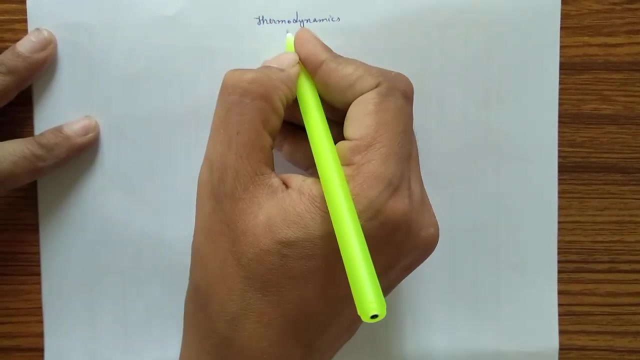 So first we will see the max distribution of thermodynamics in different examination like gate and IS, Then further we will study the entire syllabus of thermodynamics. So first we are studying with thermodynamics. As we can see if we classify thermodynamics- that is, max distribution of thermodynamics- in two broad categories. 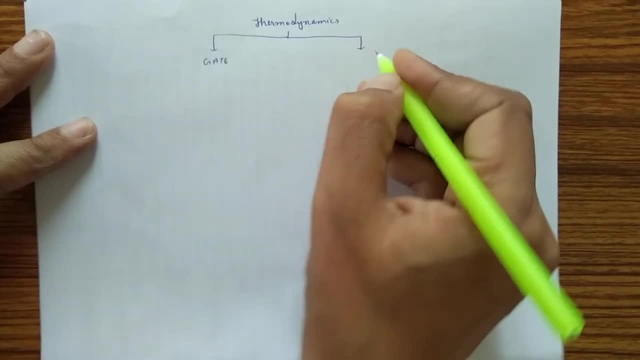 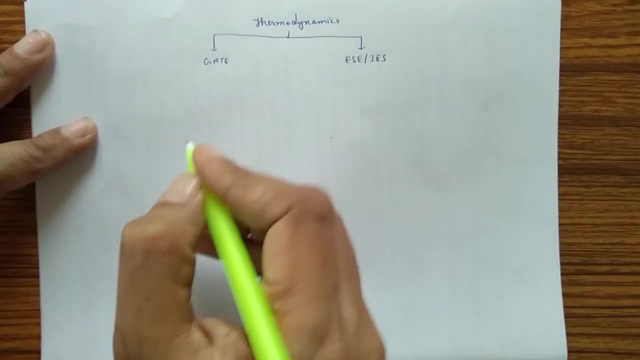 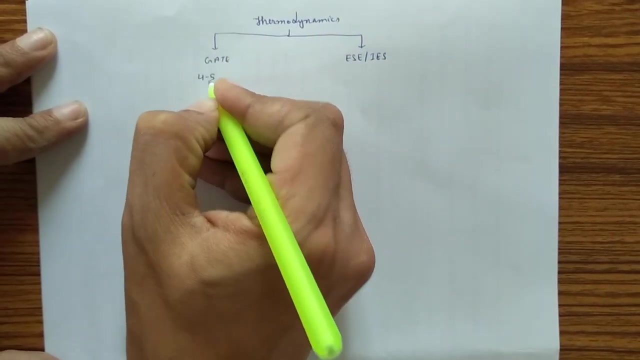 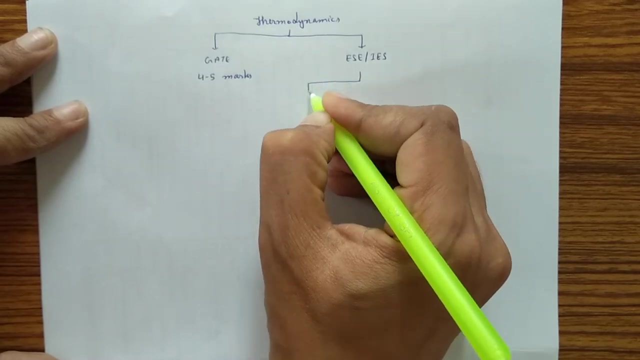 Examination, that is, gate and ESE, which was also called as IES examination. In gate it is asked for 4 to 5 marks. and IES we can classify it into two category as per objectives and conventional paper. If we see the max distribution of thermodynamics, then we can classify it into two categories. 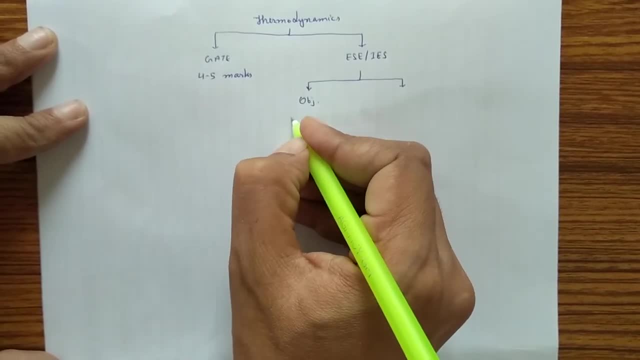 So first we will study the max distribution of thermodynamics. So first we will study the max distribution of thermodynamics. In gate. it is asked for 24 marks and IES. we can classify it into two category as per objectives and conventional paper. 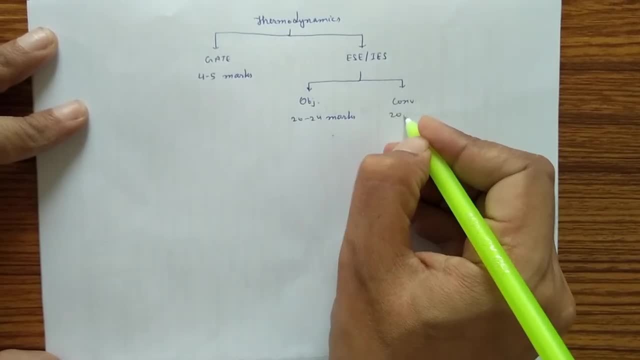 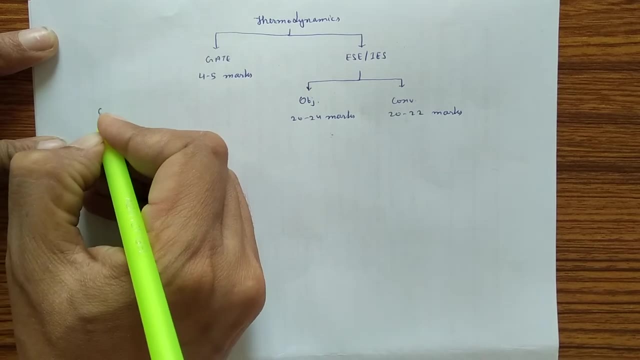 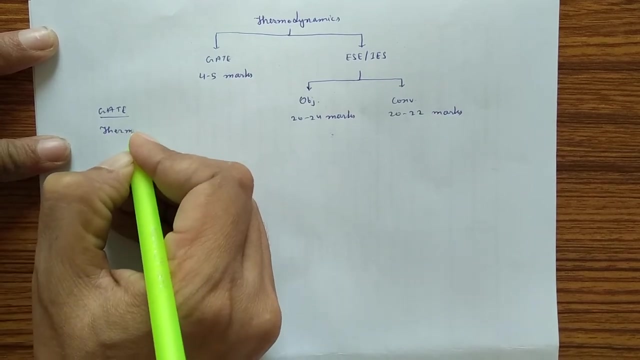 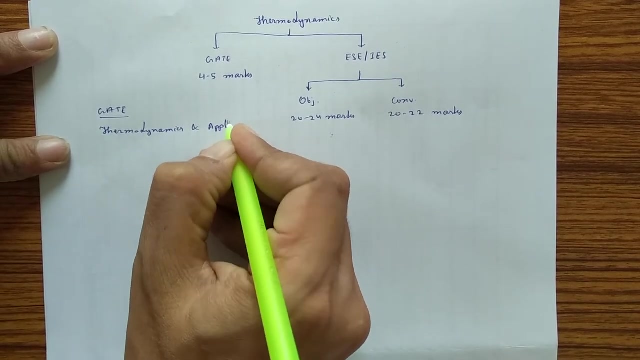 So first we will study the max distribution of thermodynamics, if we consider for gate's, then in case of thermodynamics. So first we will study the price of thermodynamics. So first we will study the price of thermodynamics and applications. 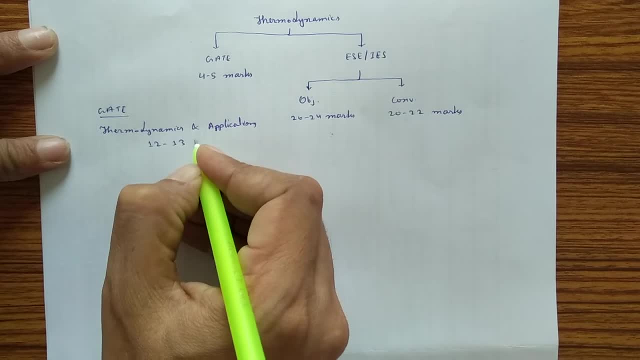 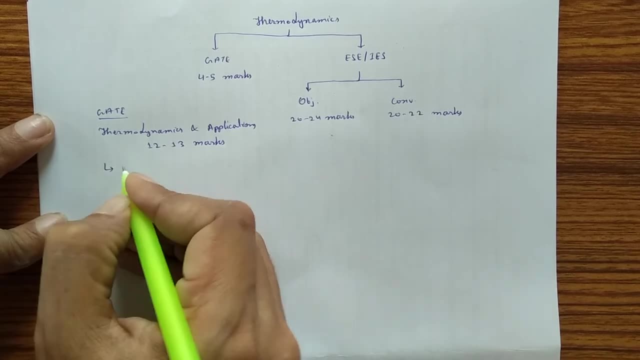 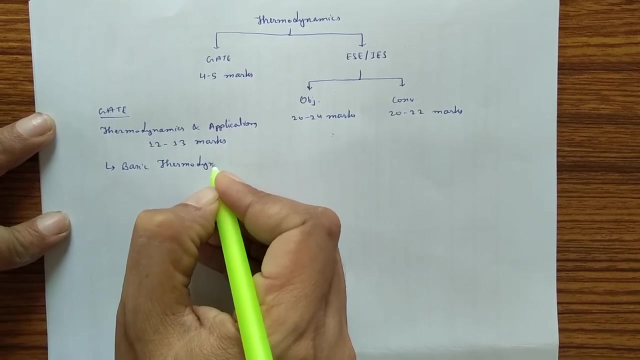 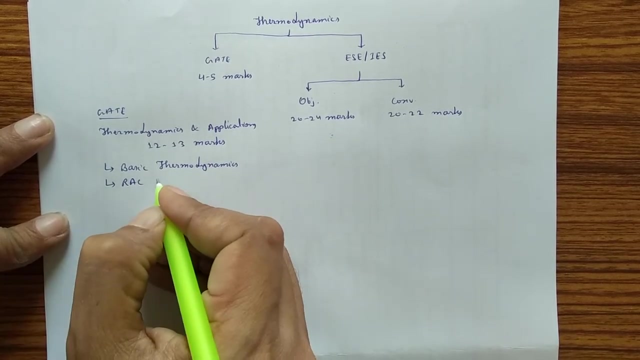 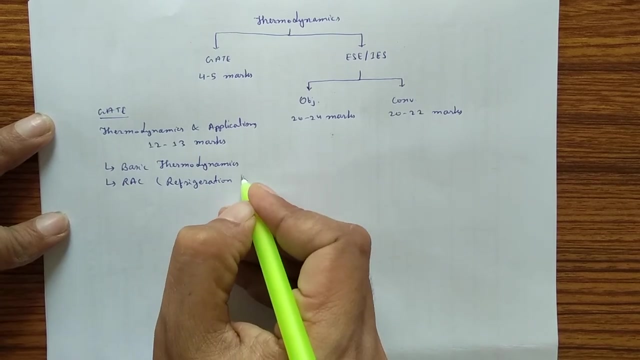 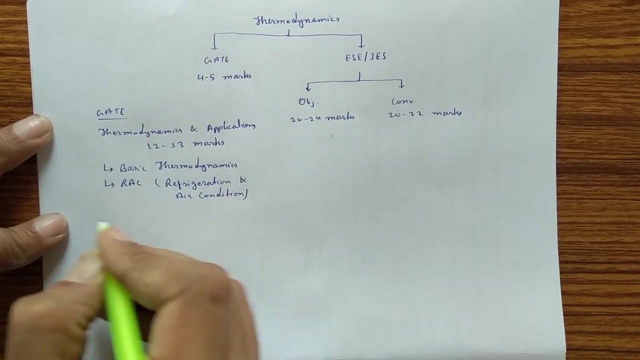 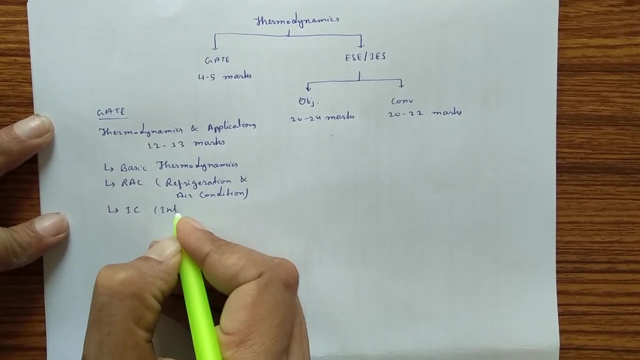 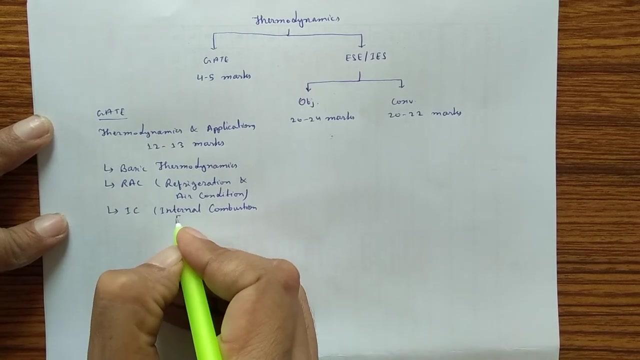 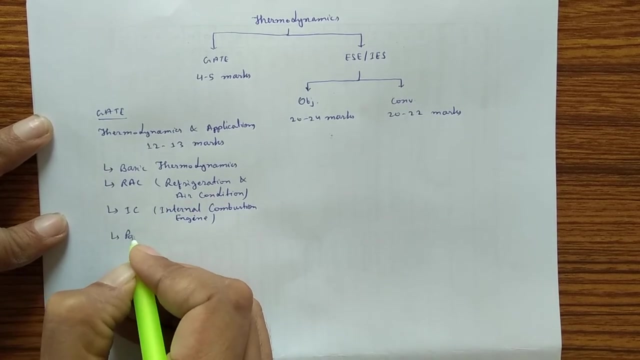 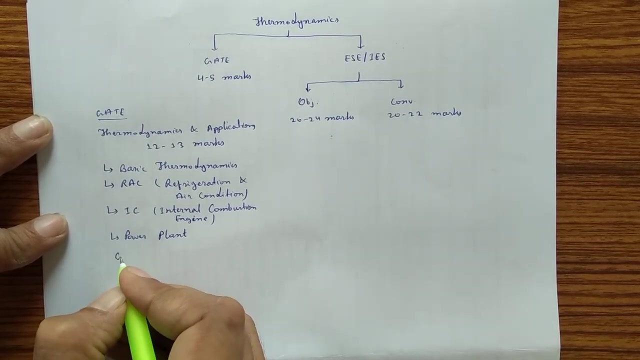 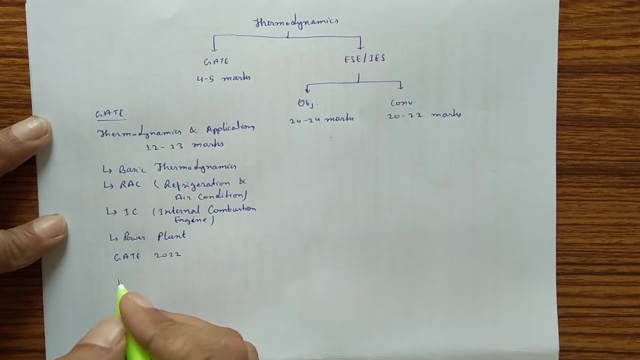 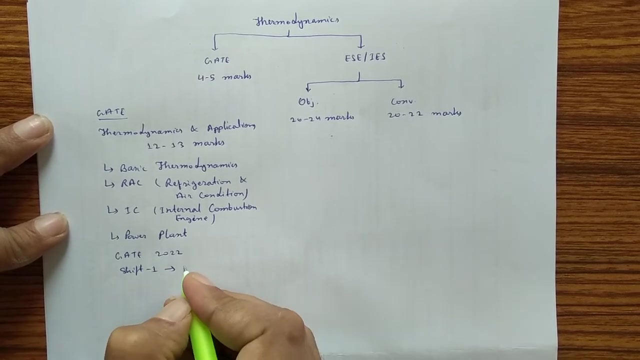 it is asked for 12 to 13 marks in this includes basic thermodynamics, RAC, that is, refrigeration and air conditioning- IC, internal combustion engine and power plant. if we see analyze gate 2022, we see in shift 1 they have asked 3 marks. 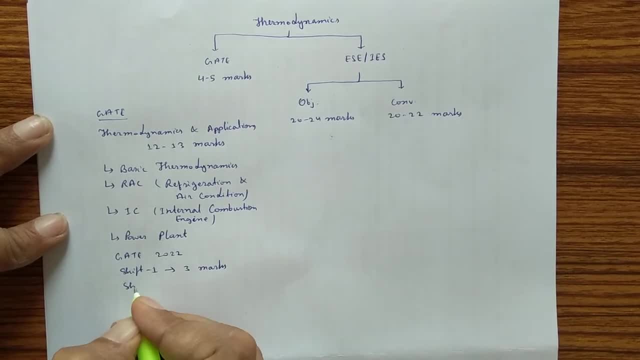 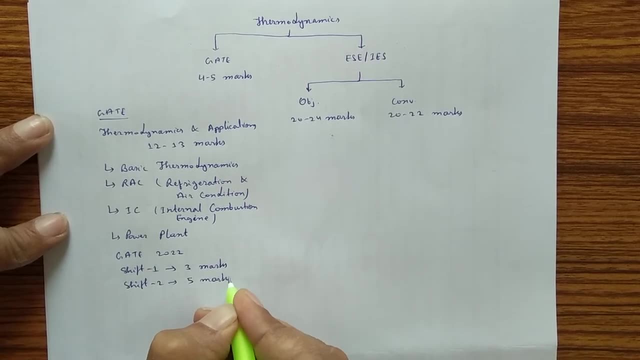 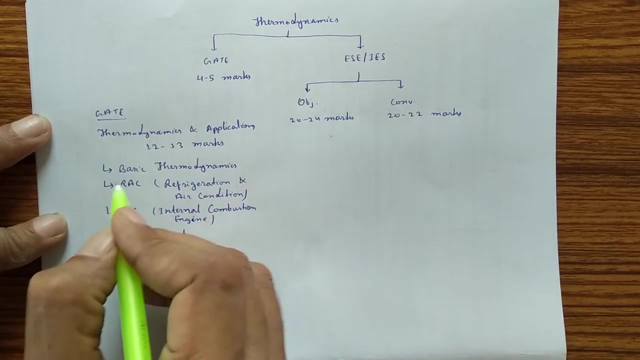 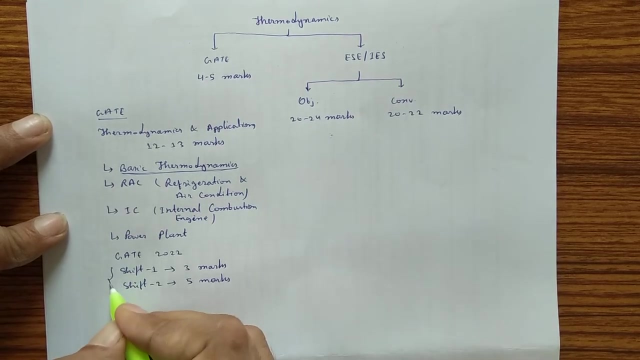 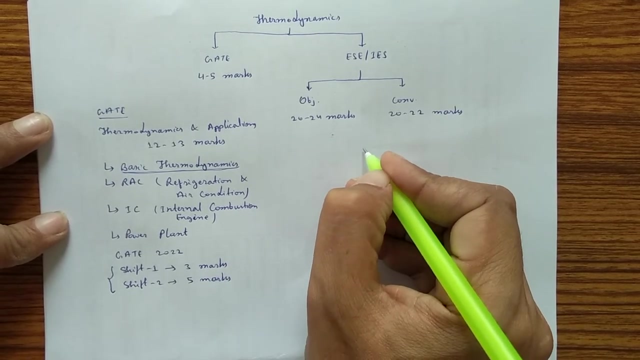 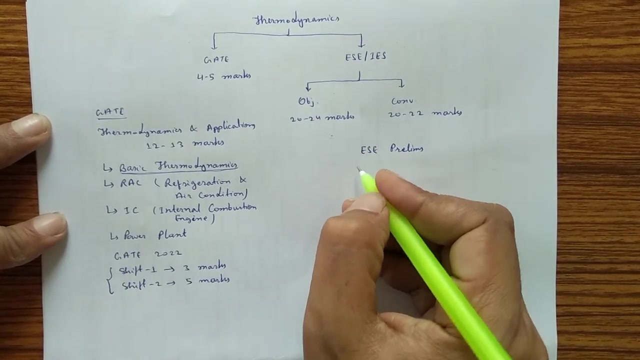 questions. and in shift 2 they have asked total 5 marks questions from thermodynamics, only from thermodynamics. that one, only this basic. I am talking about only this basic. they have asked these questions in gate 2022 if we come for IS examination. so ESE prelims. 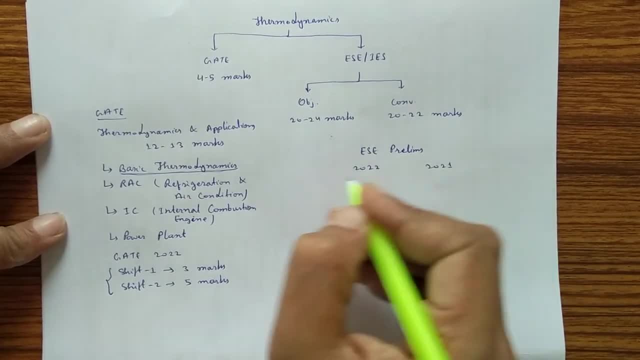 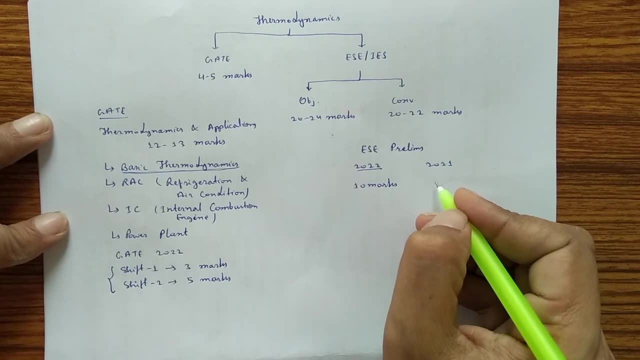 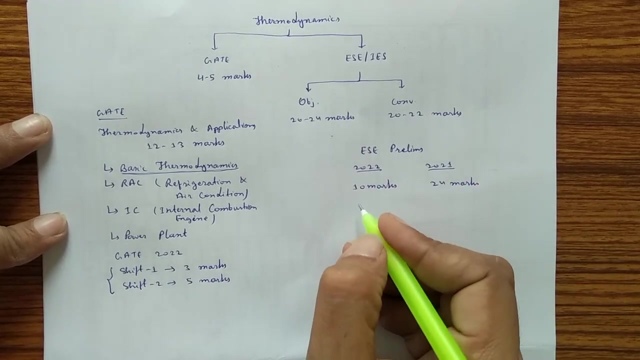 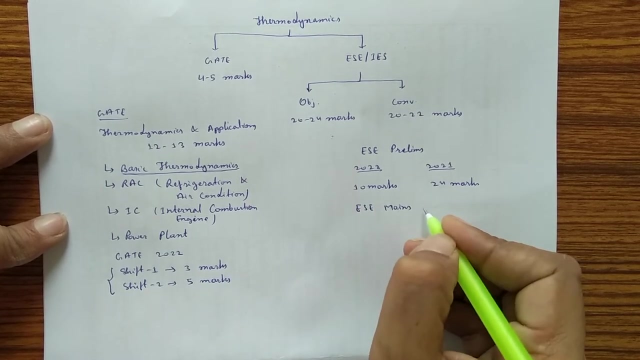 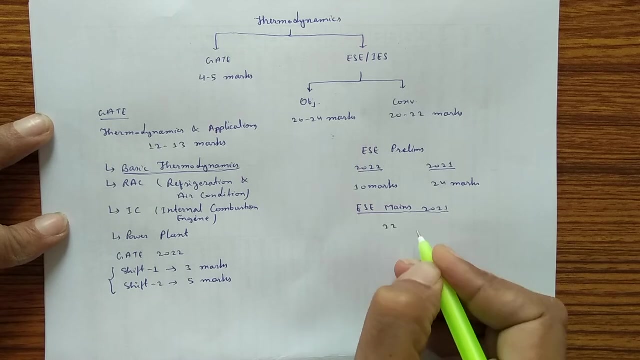 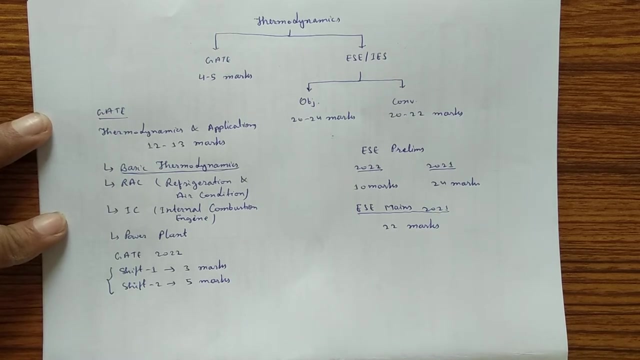 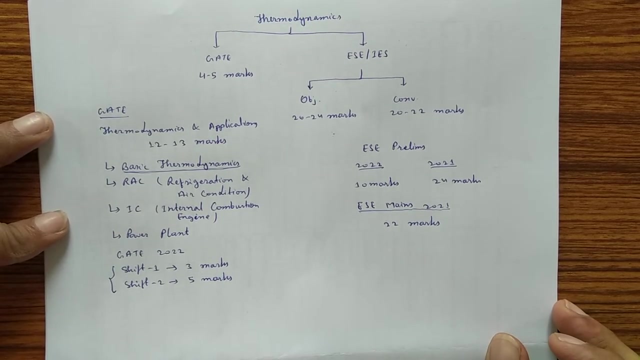 2022- 2021. in 2022 they have asked 10 marks questions and 2022 they have asked 24 marks. if we come for ESE means 2021 they have asked 22 marks questions. this is the marks distribution of thermodynamics and these two exam missions. 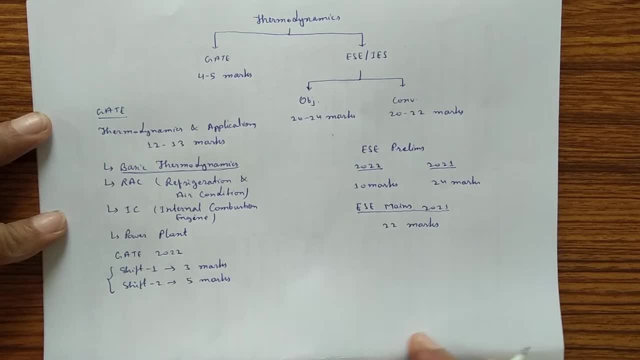 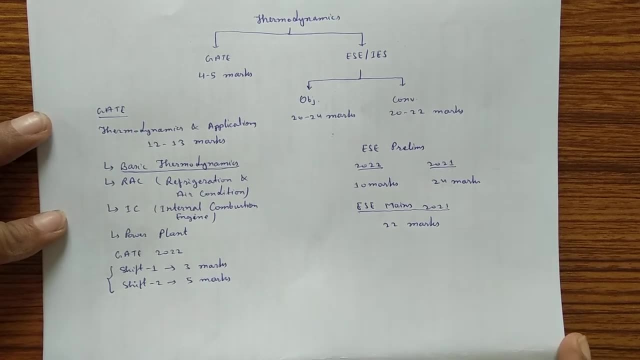 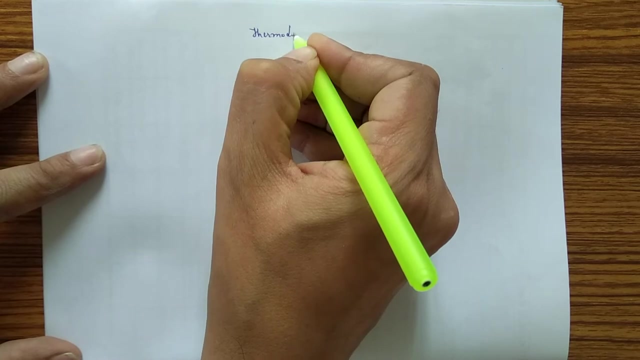 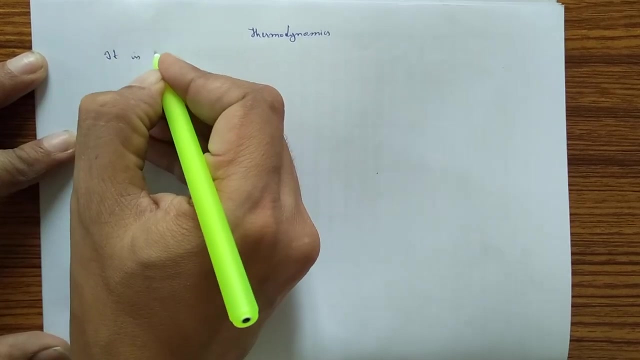 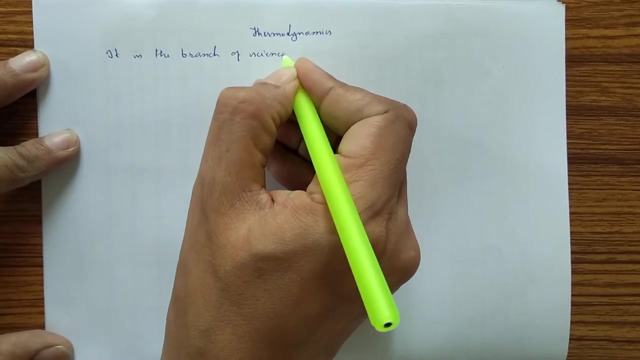 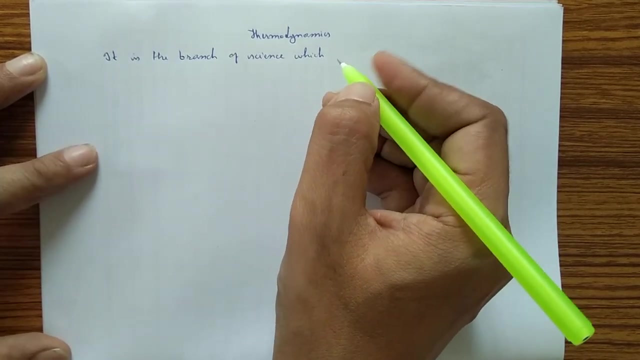 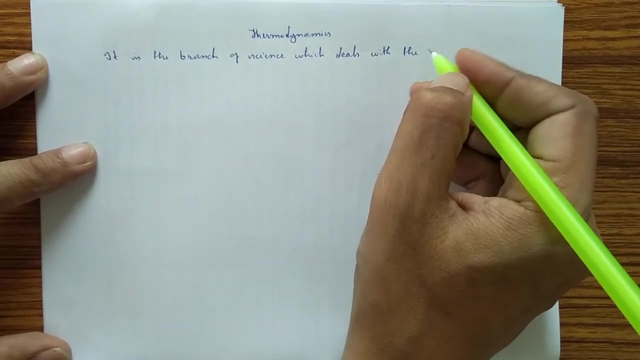 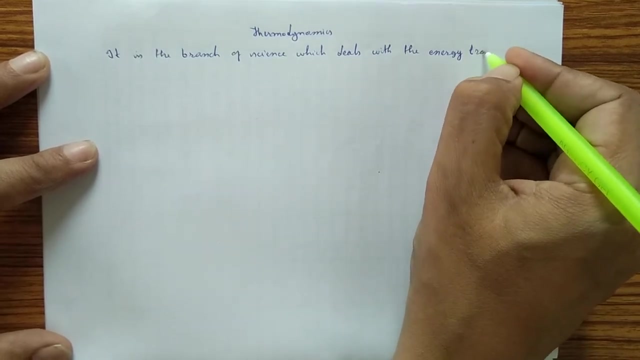 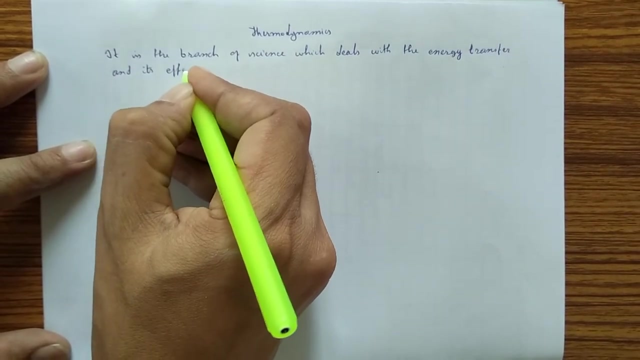 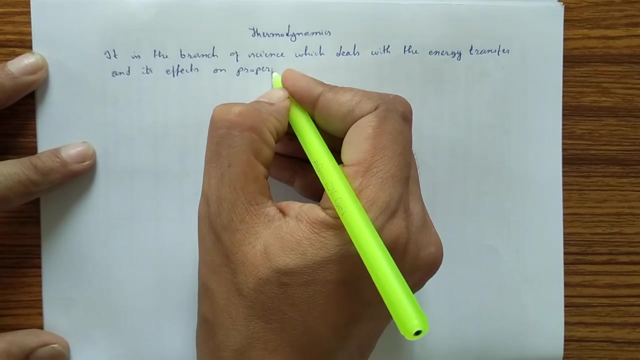 we will discuss on different examinations also. now we will start with the basic concepts of thermodynamics. thermodynamics, it is the branch of science. it is the branch of science. it is the branch of science which deals with the energy transfer and its effects and its effects on properties. 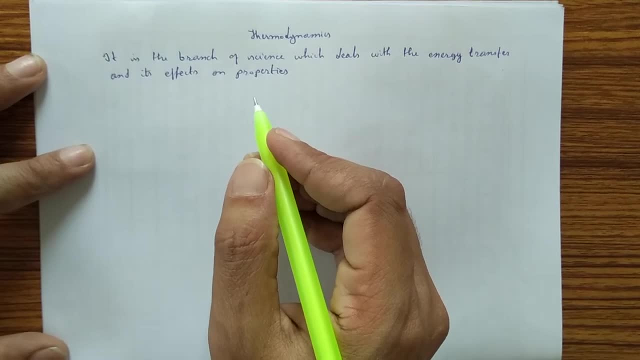 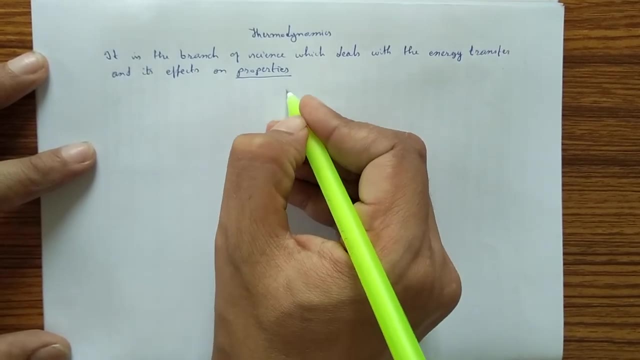 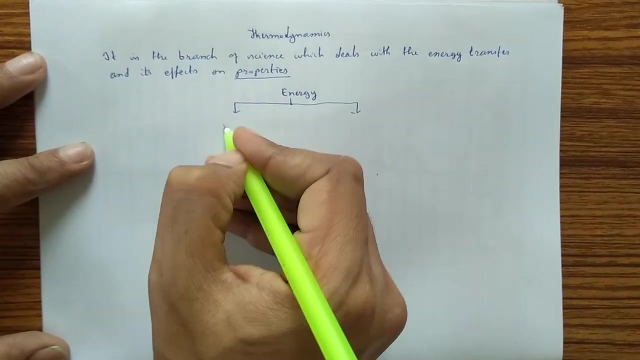 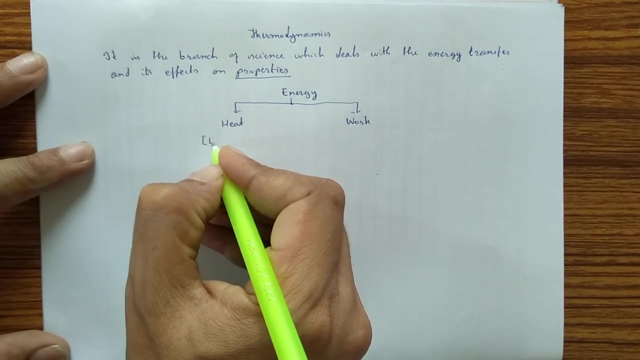 so it is mainly the science of energy transfer and its effects on properties. we will discuss about properties first. we see energy. here we will take two forms of energy. one is heat and other is work. heat is considered as low grade form of energy and work as high grade form of energy. 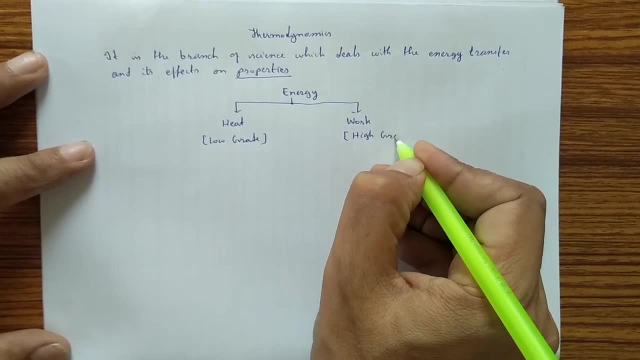 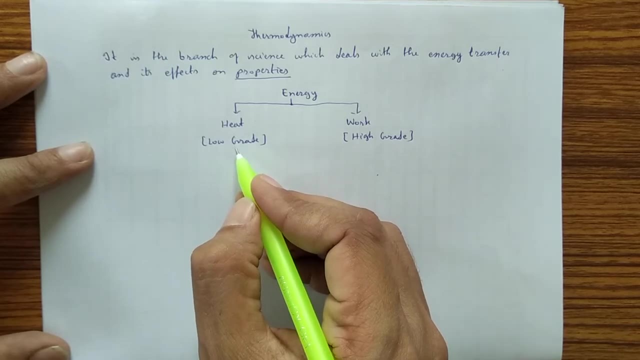 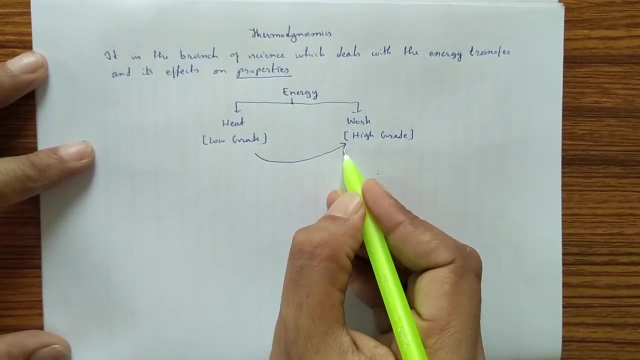 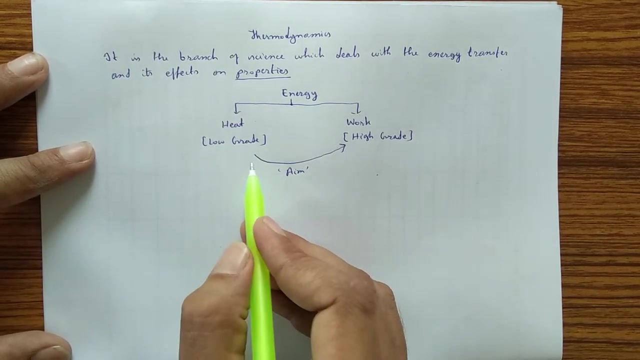 the aim of thermodynamics is to convert this low grade form of energy, which is heat, to high grade form of energy work in an efficient manner. so what is the aim of thermodynamics? the aim of thermodynamics? the aim of thermodynamics, is to convert low grade form of energy- heat- into high grade form of energy work. 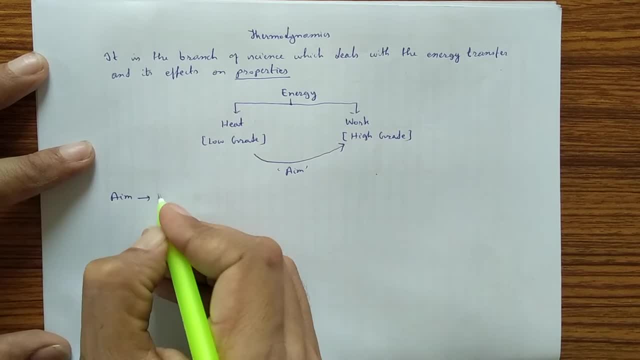 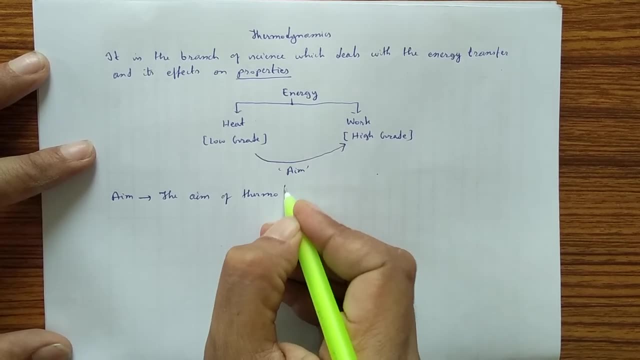 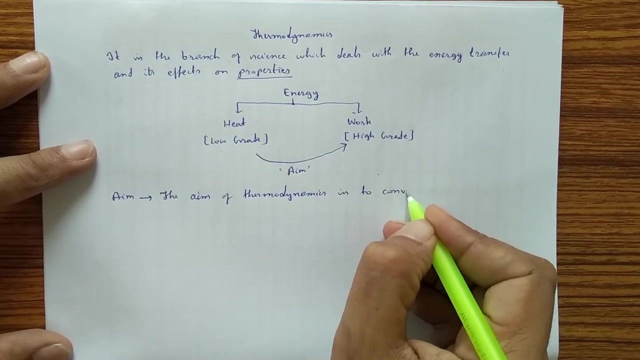 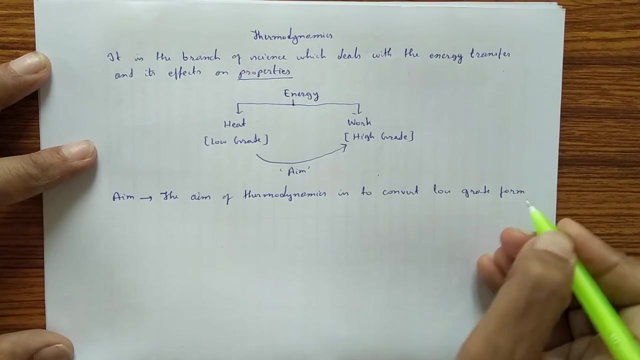 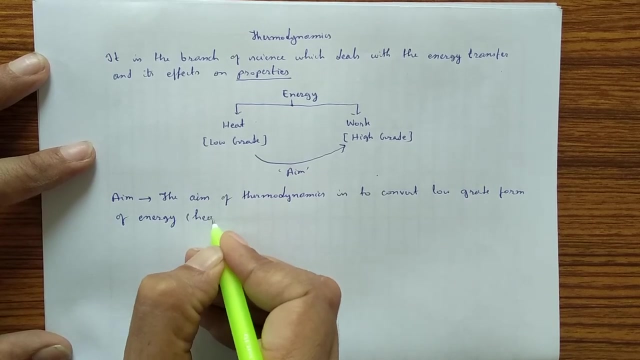 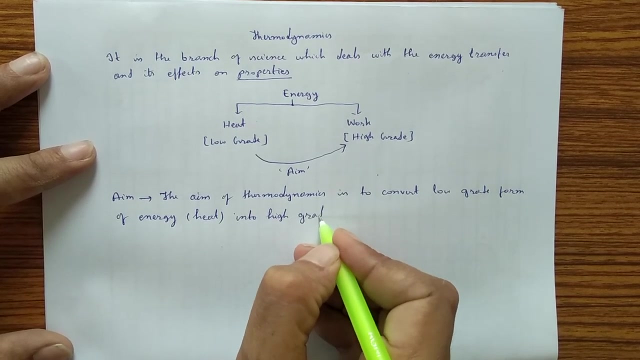 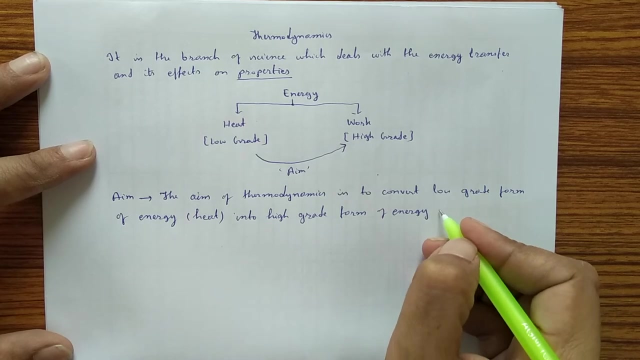 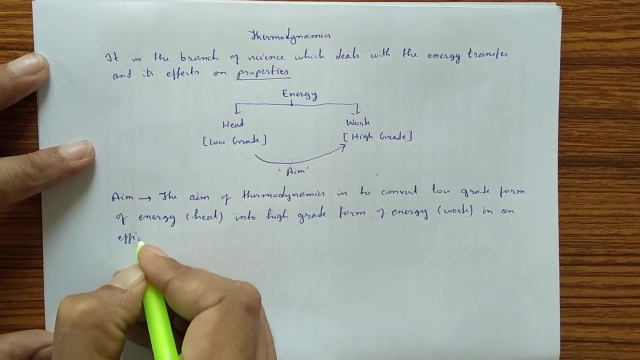 so we can write this: the aim of thermodynamics is to convert low grade is to convert energy- heat into energy, free form of energy, which is heat, into low grade form of energy and energy is to convert energy into high grade form of energy in an efficient manner. 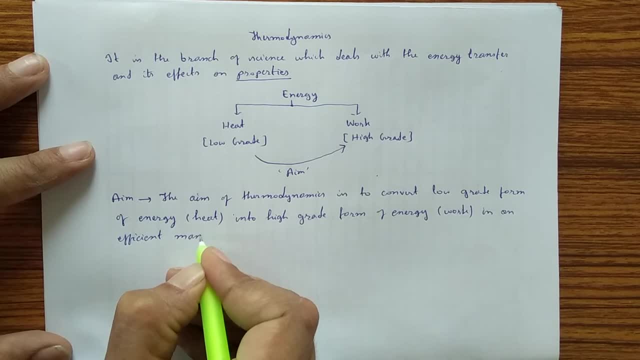 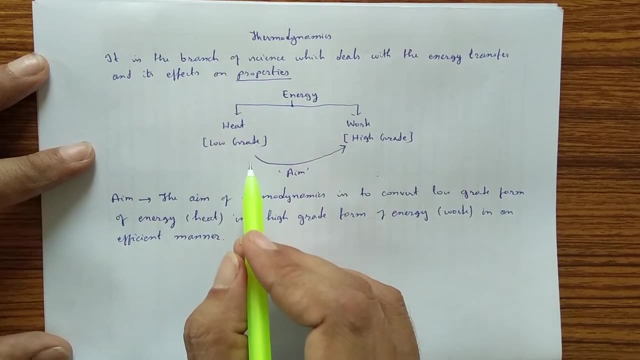 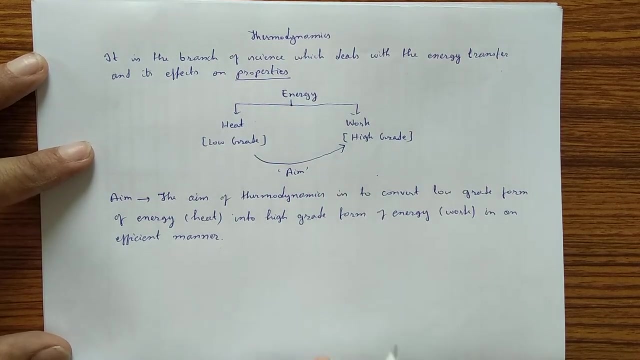 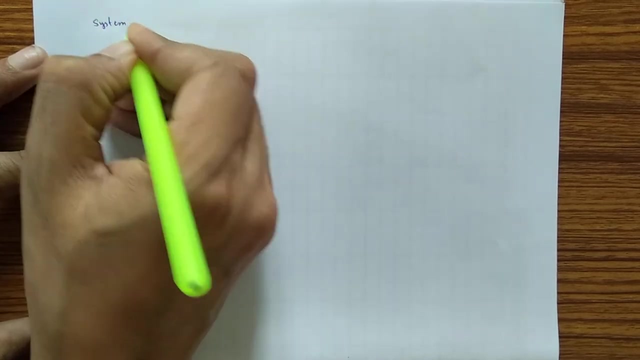 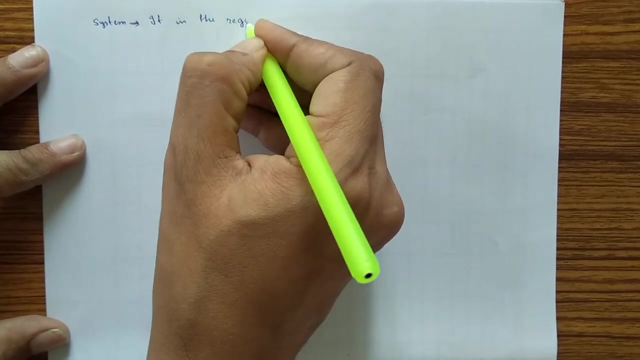 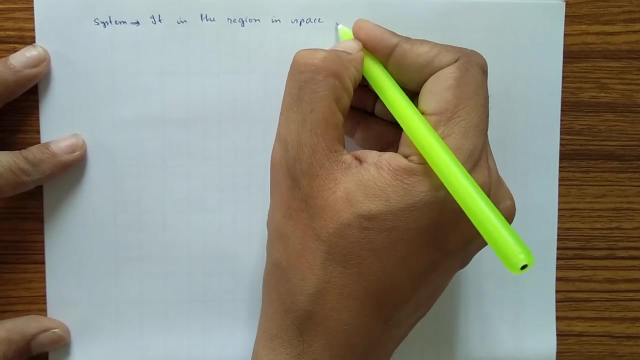 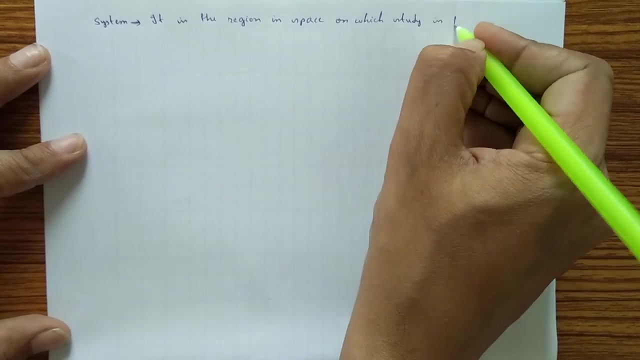 so the aim of thermodynamics is to convert this heat to work in an efficient way, that is, with high efficiency. now we will study with basic definitions and terms in thermodynamics, so let's start that system. it is the reason and space on which study is focused. 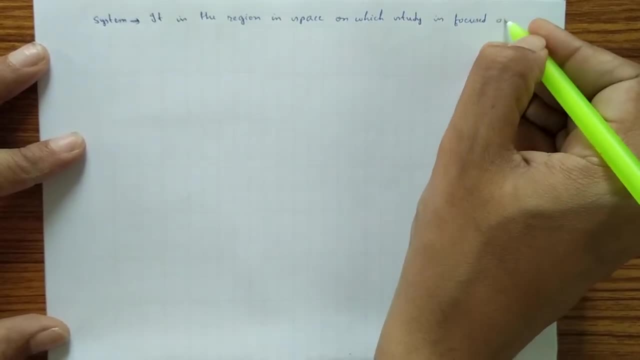 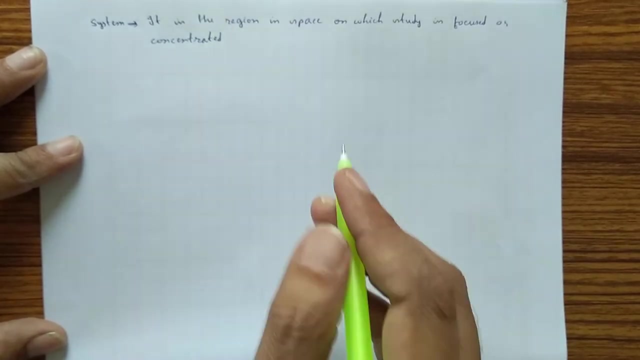 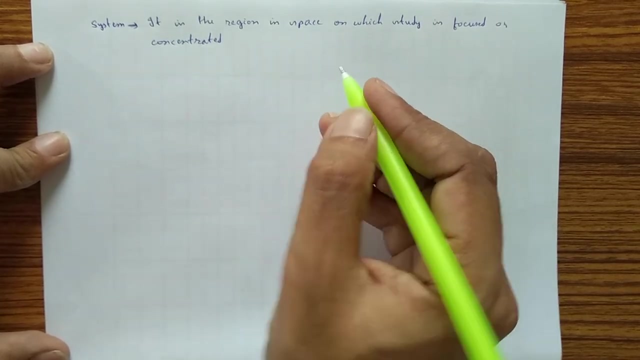 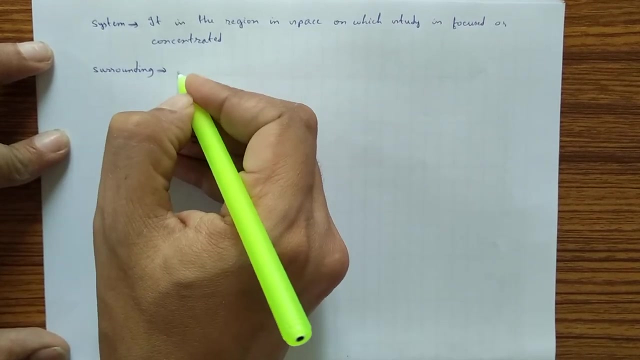 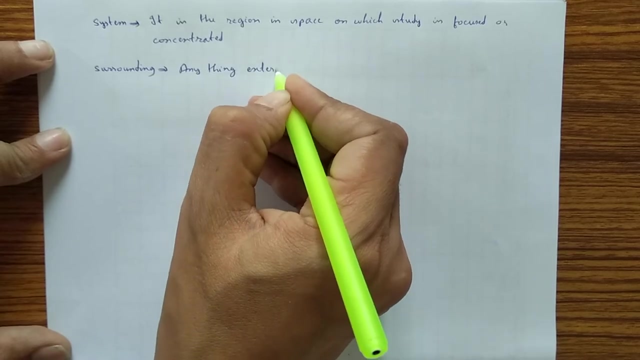 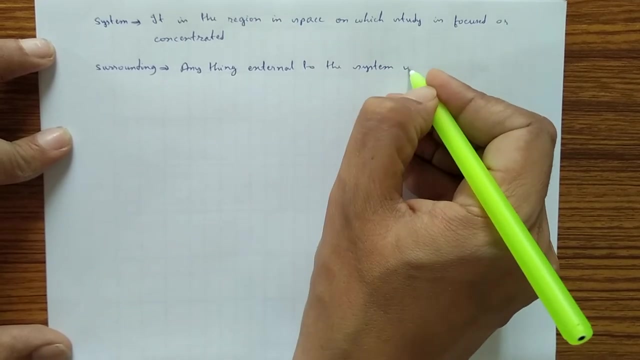 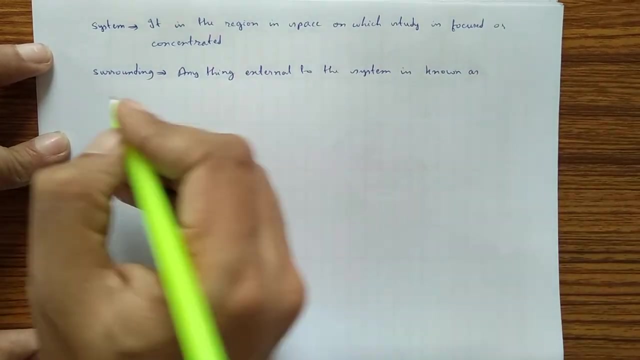 on or concentrated. so system is the reason in space on which our study is focused or concentrated. the other term is surrounding anything external to the system on which our study is focused or concentrated. the system is known as subscribe and run on our linear independence bumper on Canadians. 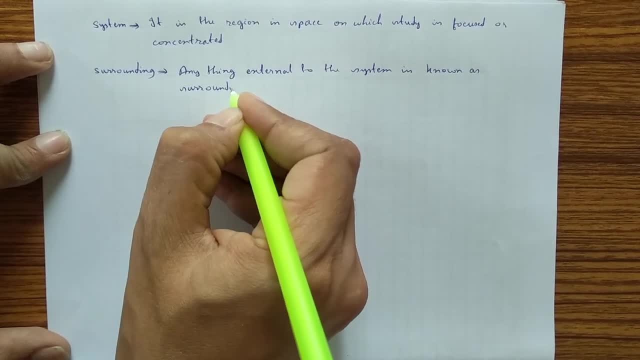 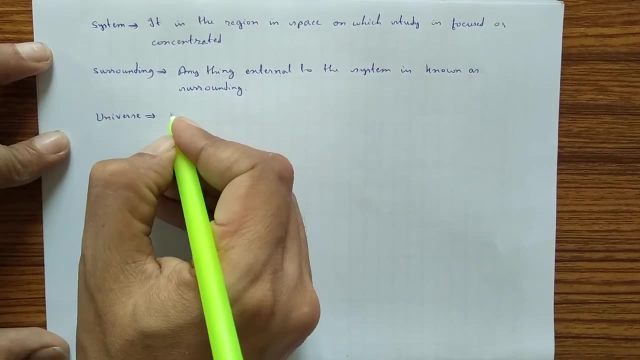 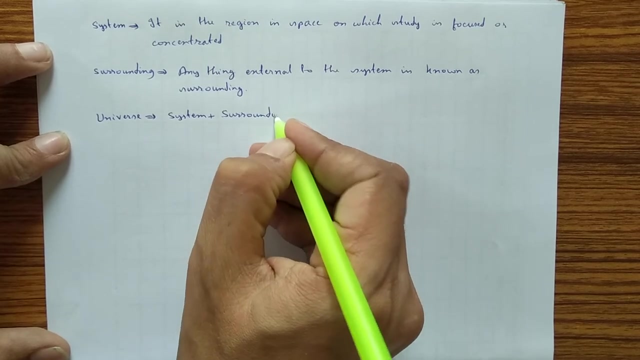 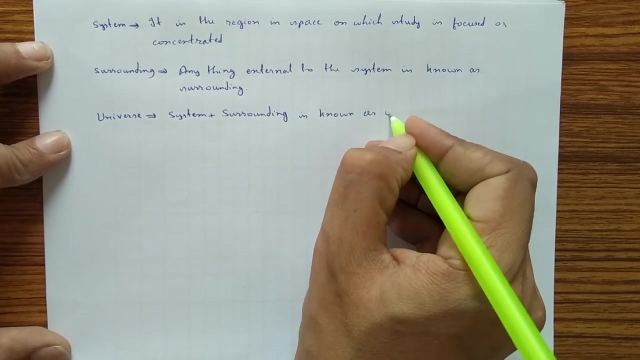 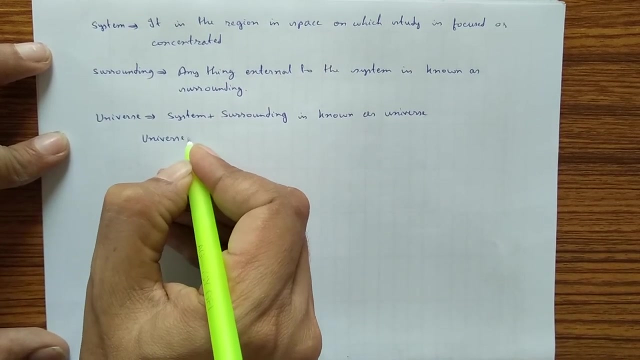 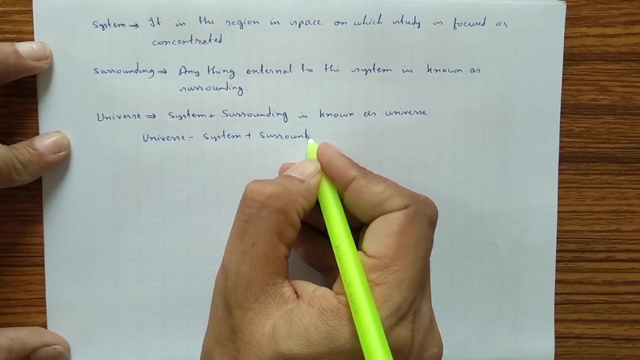 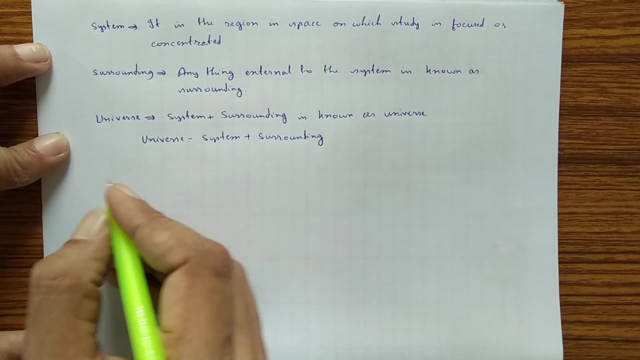 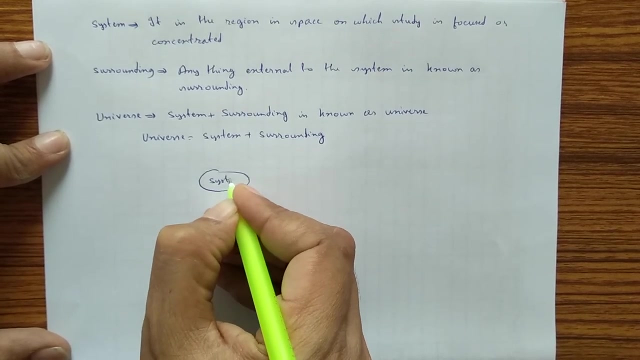 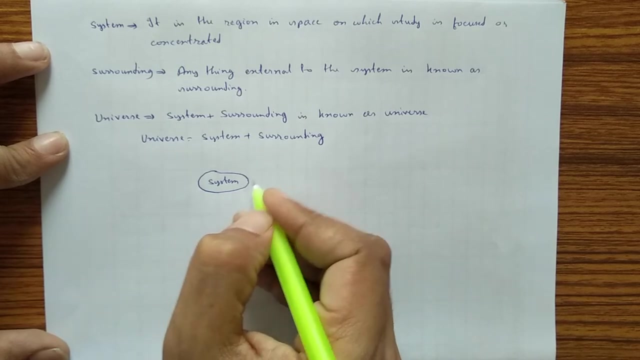 on the Internet is known as tür iv universe of US. the reason for collaborating with programs, system surrounding, is known as universe, so we can write universe equal to system plus surrounding. if it is our system, then our state is based on the system only. everything external to the system is our. 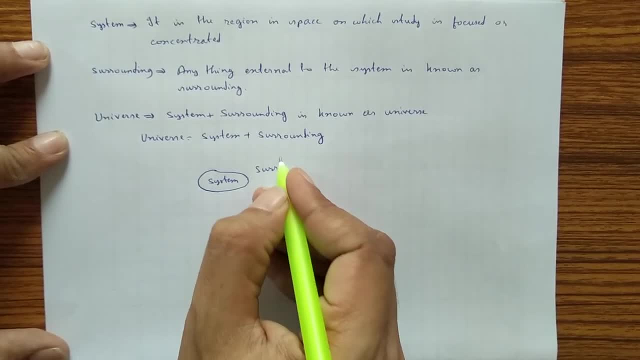 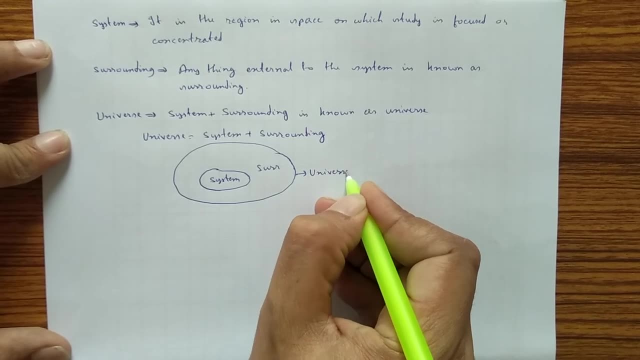 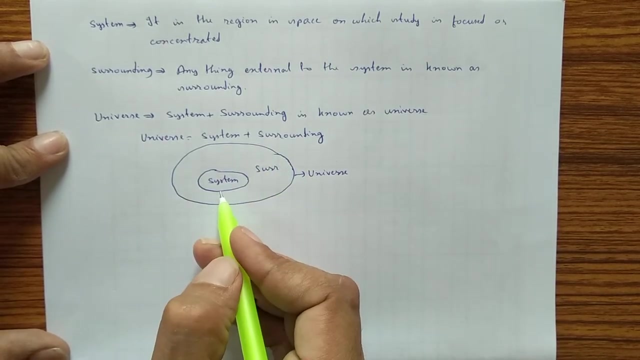 surrounding. and if we combine system plus surrounding, this whole system is our surrounding, as will be considered as universe. so system is on which our study is based. whatever we want to study, that is considered as system and other than other things which is out of the systems or surroundings. and if we combine the, 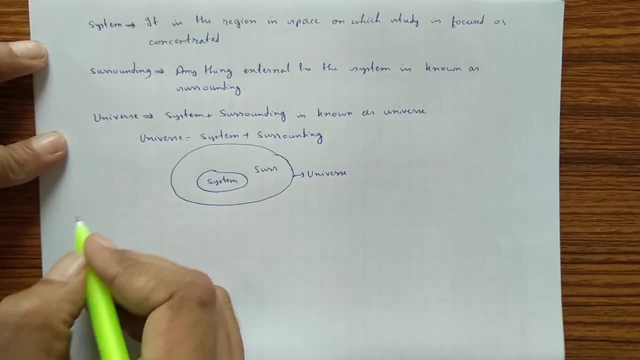 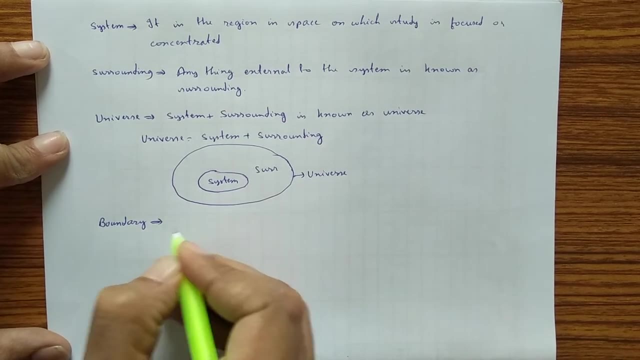 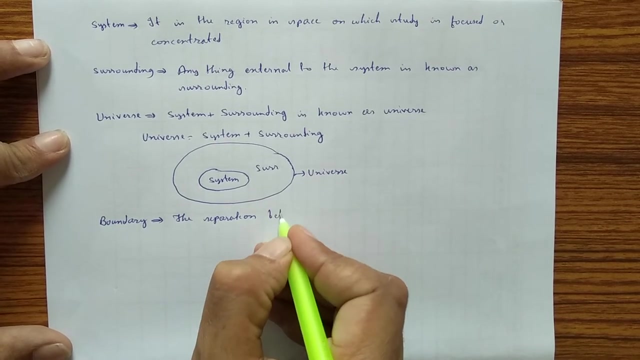 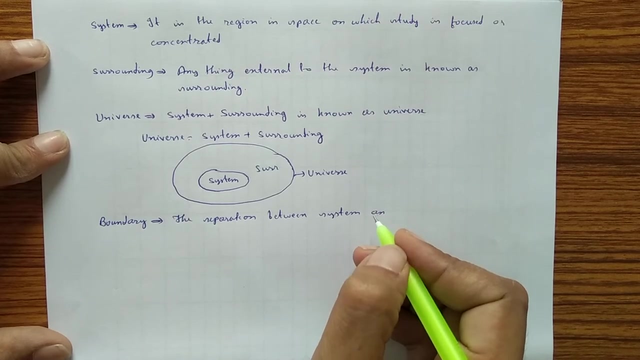 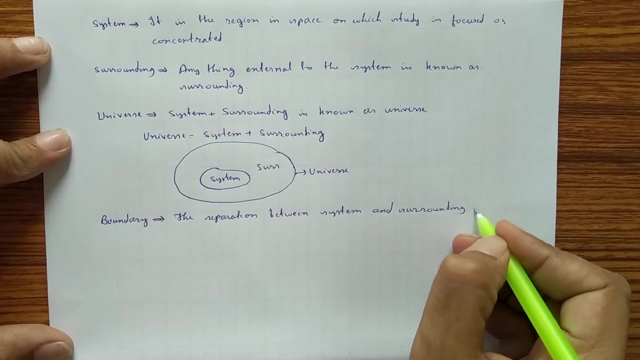 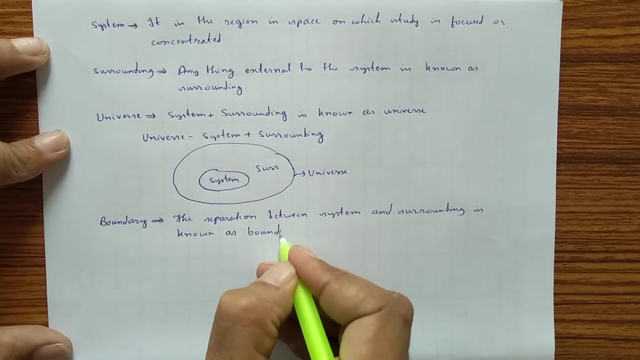 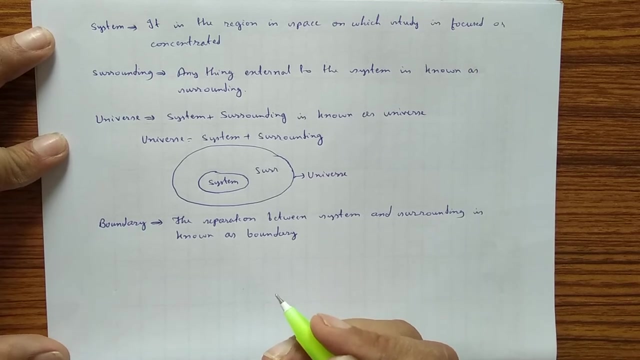 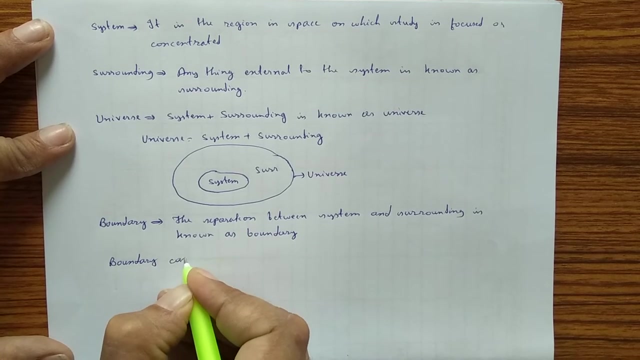 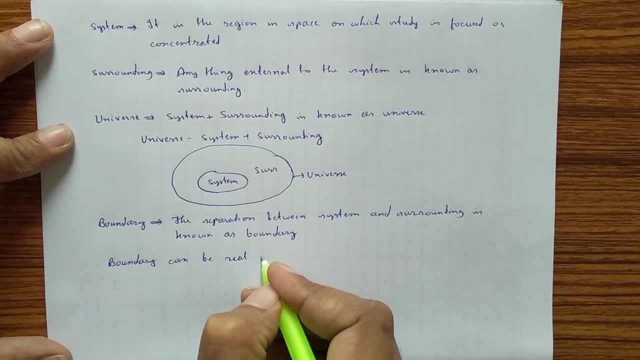 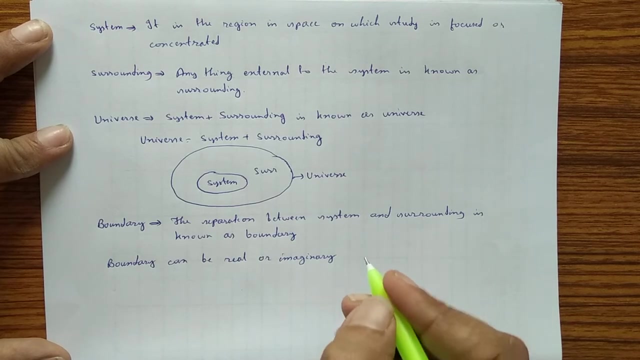 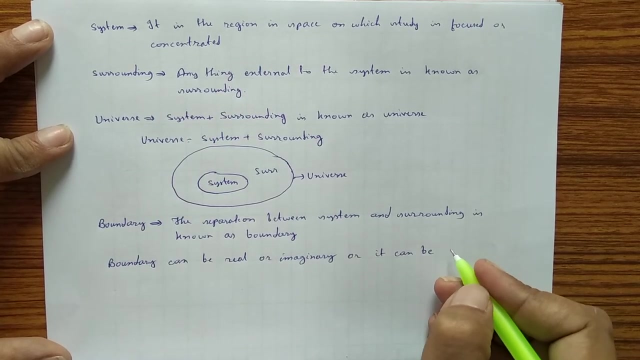 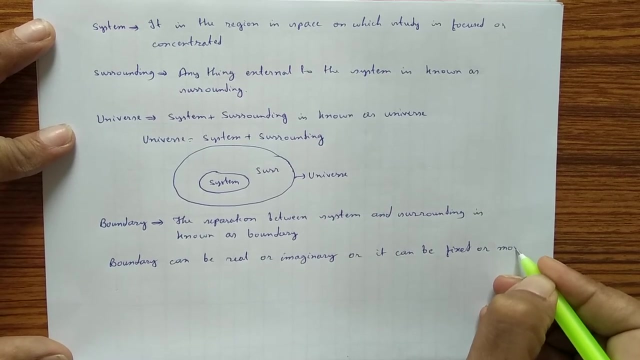 CA system plus rounding. that is called as universe boundary, the separation between system and surrounding is known as boundary. so boundary is the separation between system and surrounding. so boundary can be can be real or imaginary, or it can be fixed or movable. so we will see the examples of boundaries. 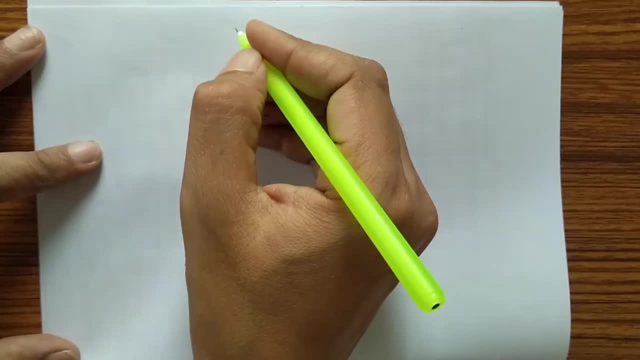 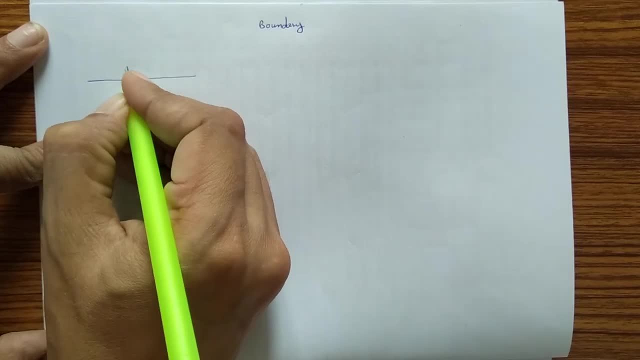 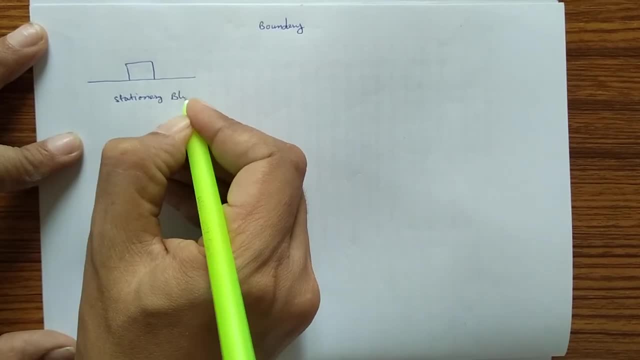 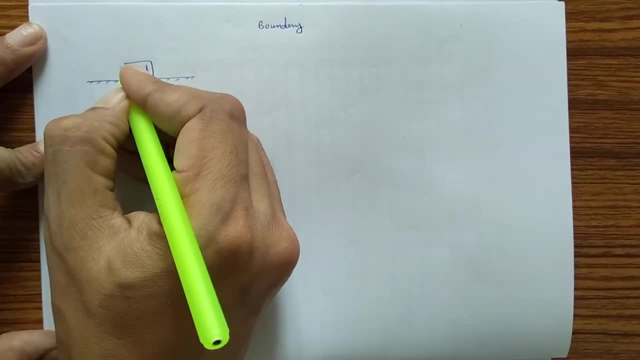 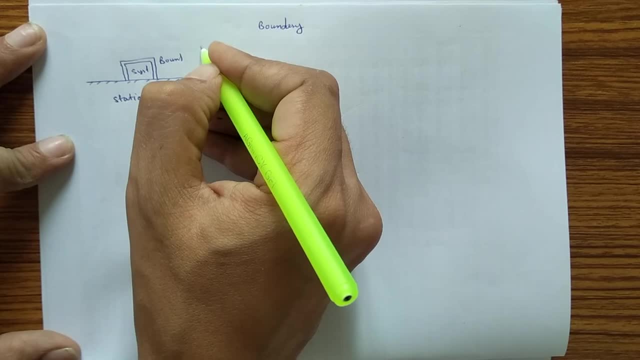 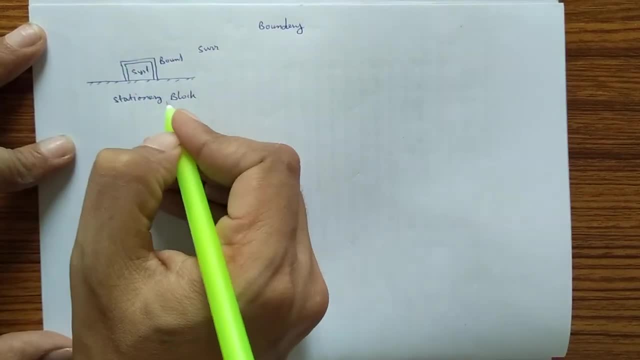 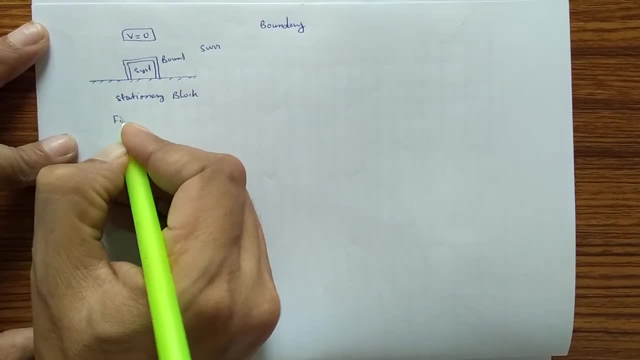 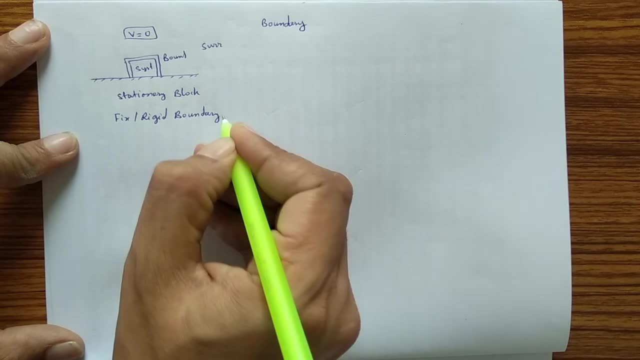 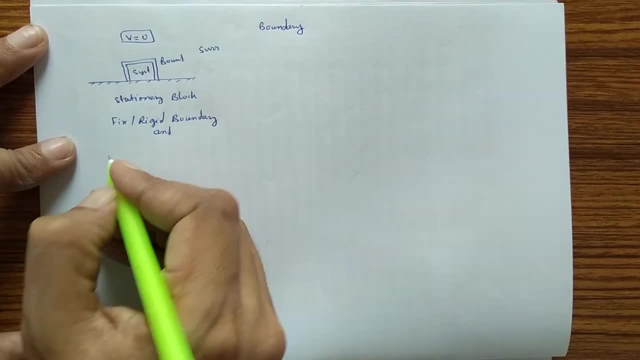 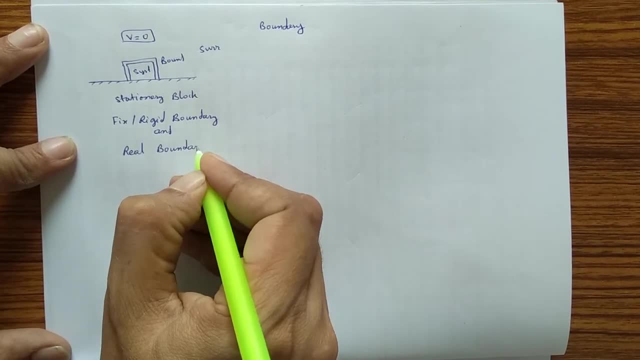 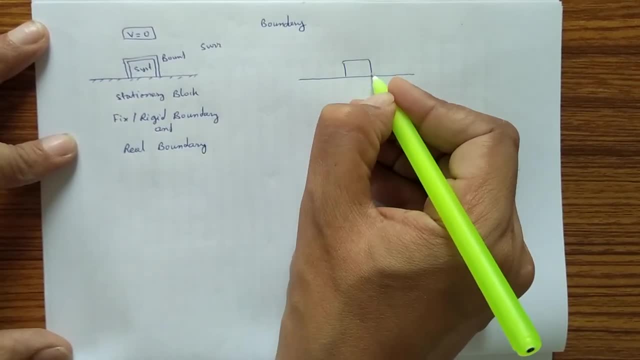 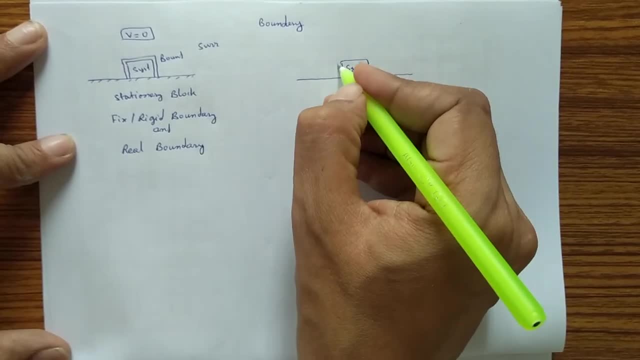 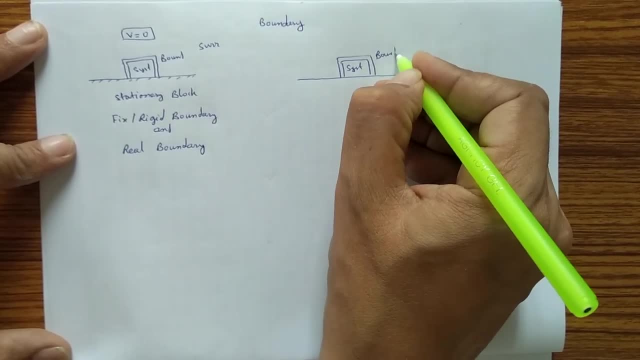 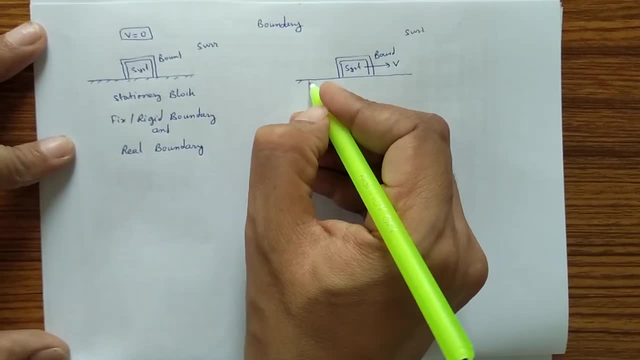 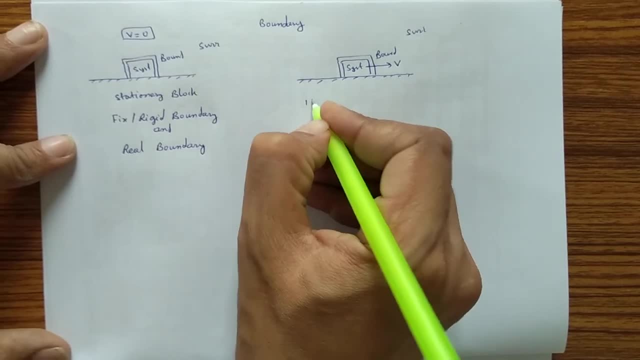 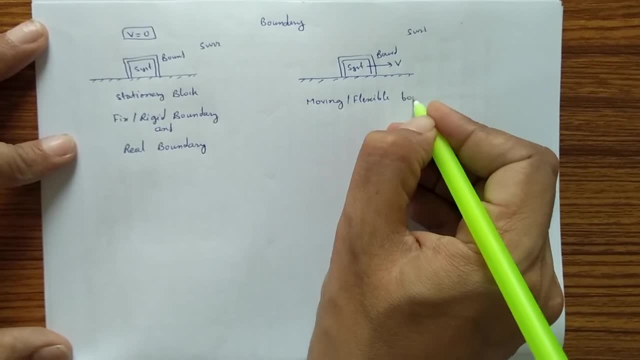 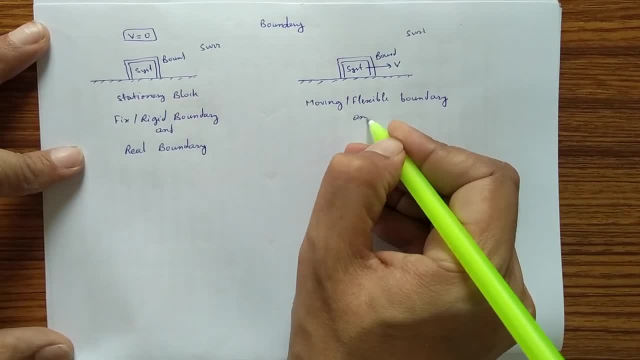 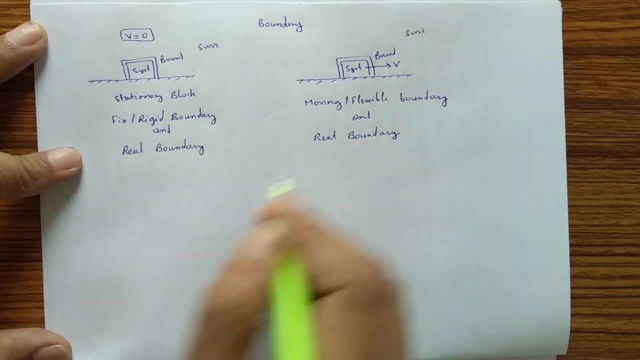 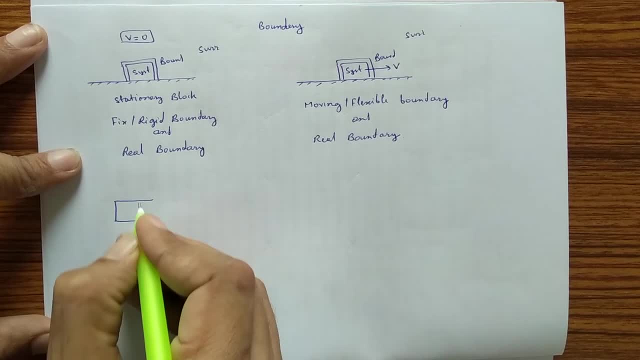 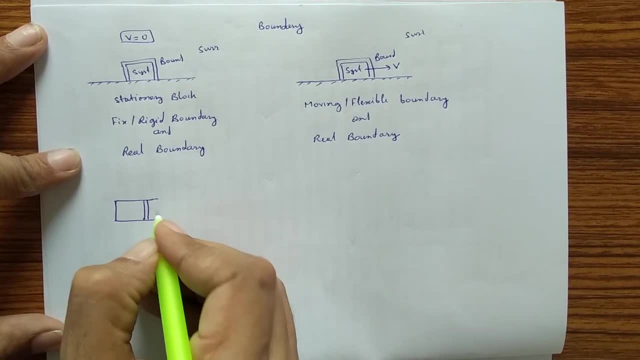 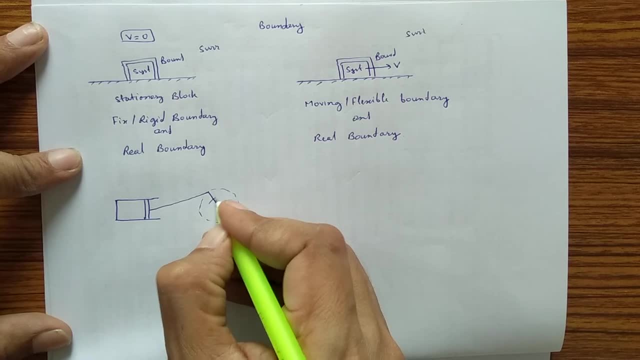 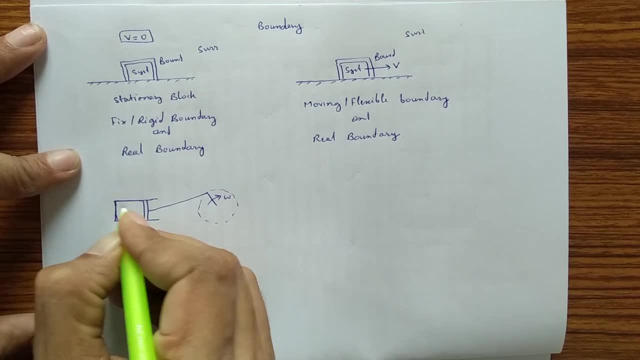 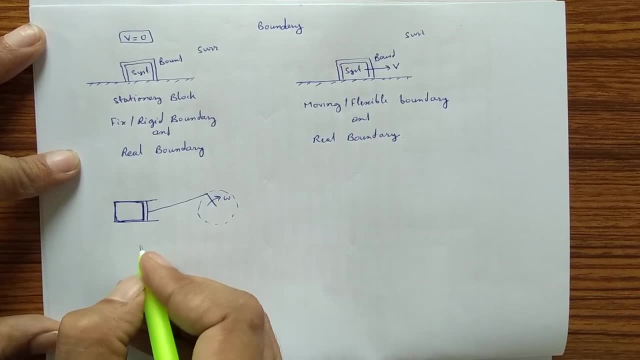 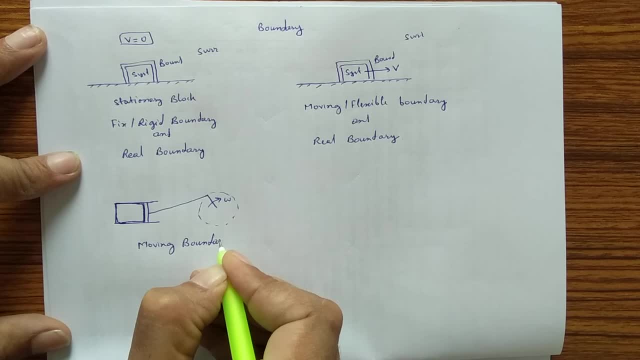 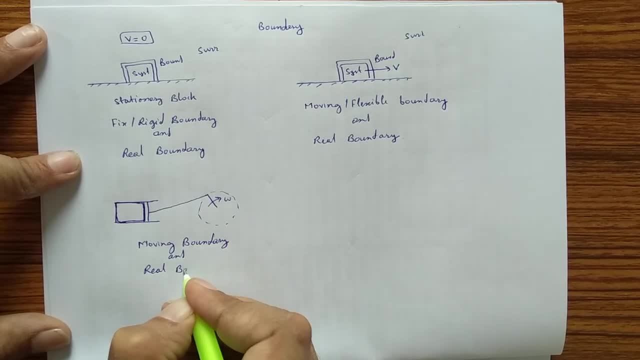 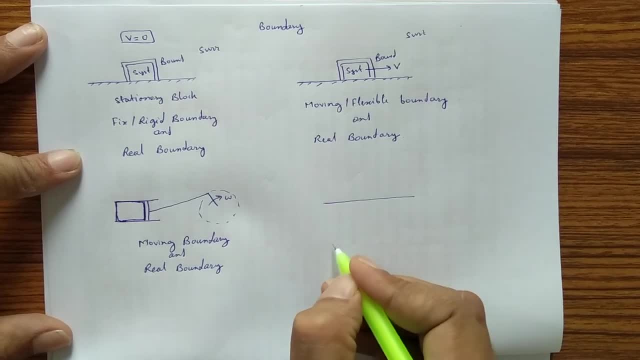 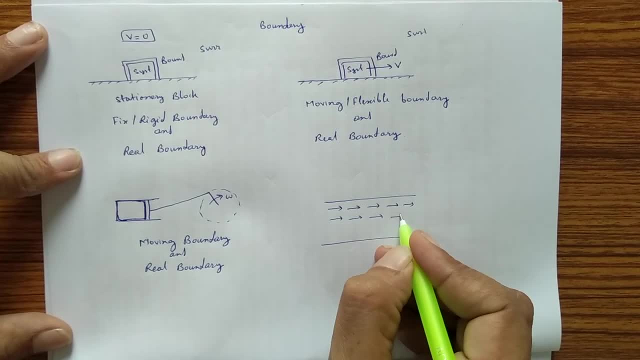 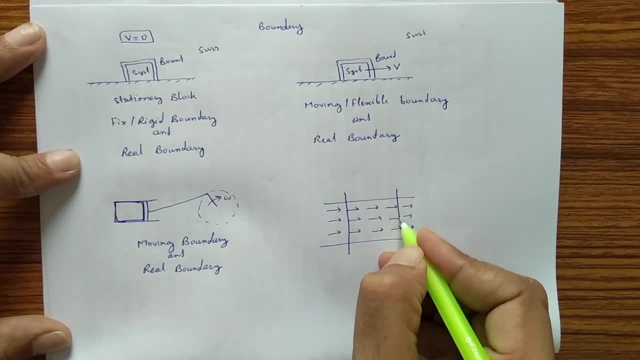 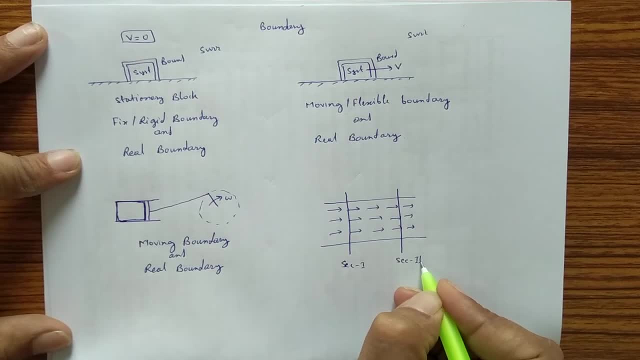 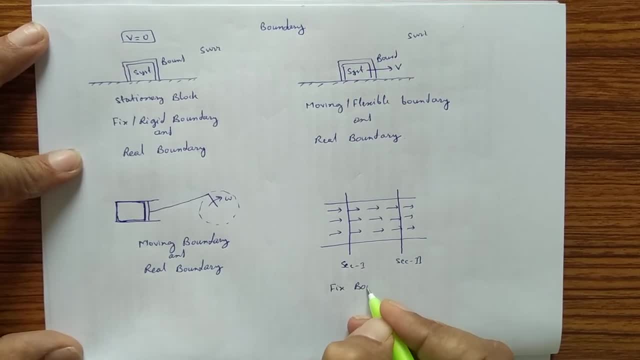 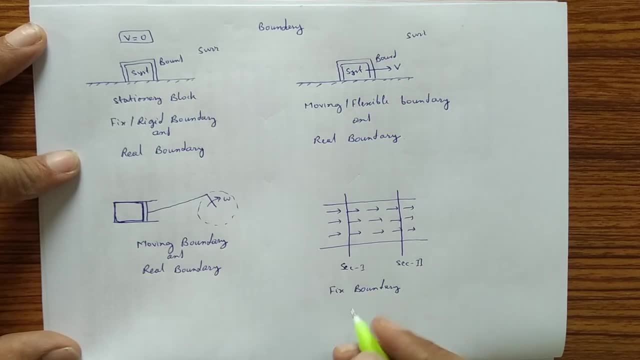 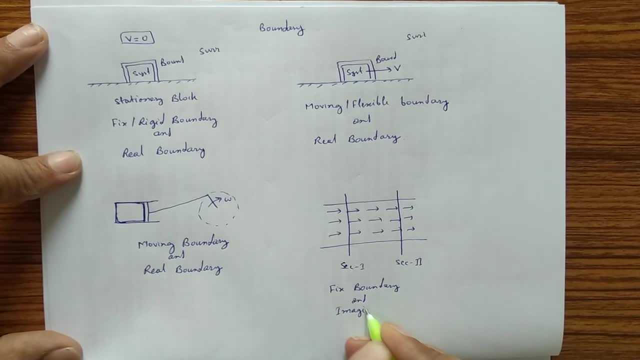 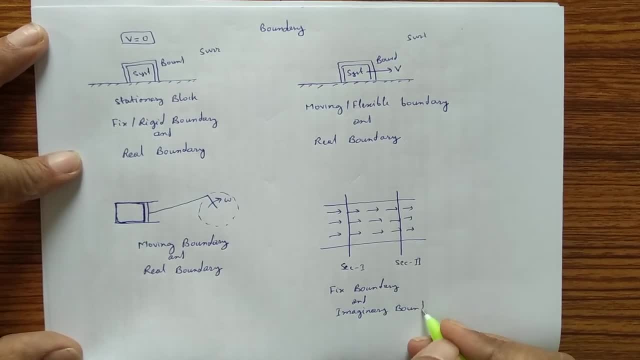 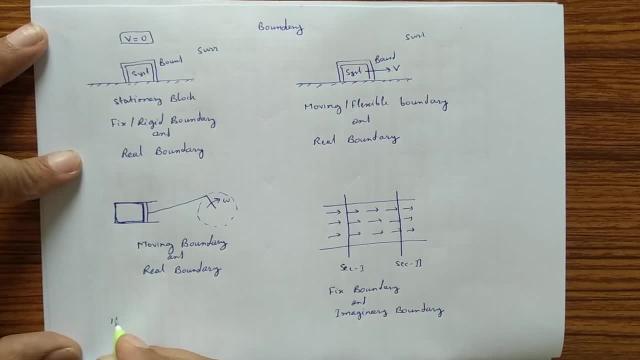 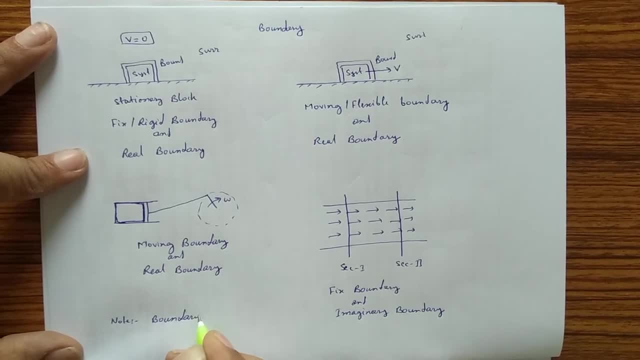 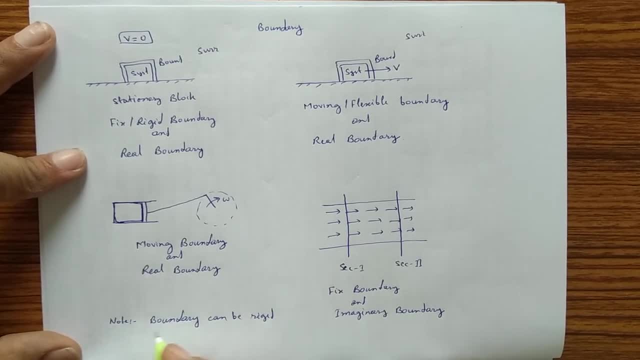 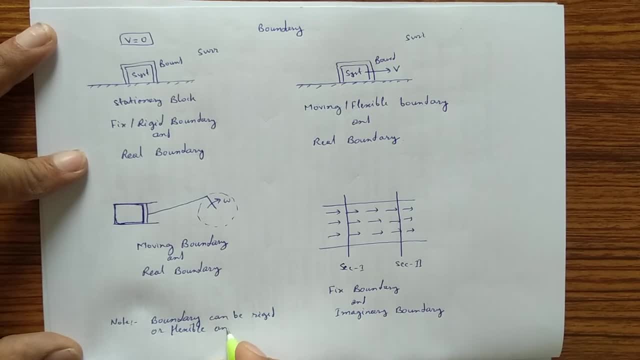 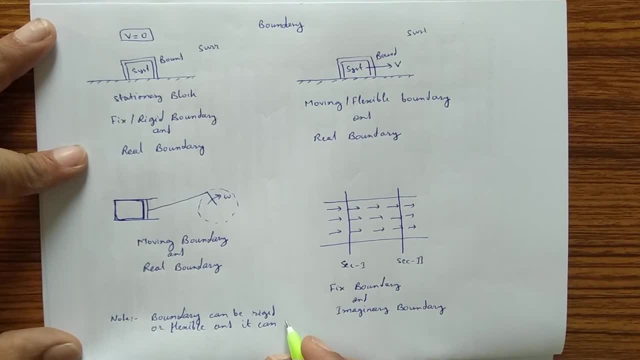 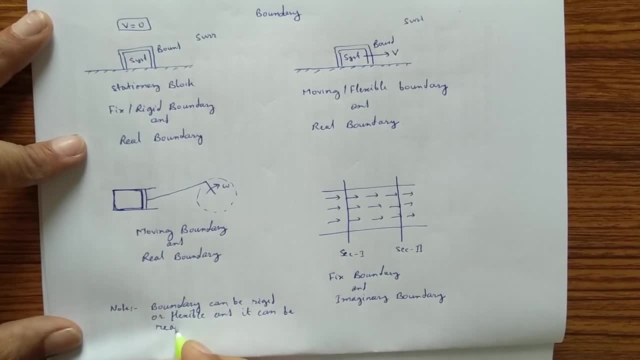 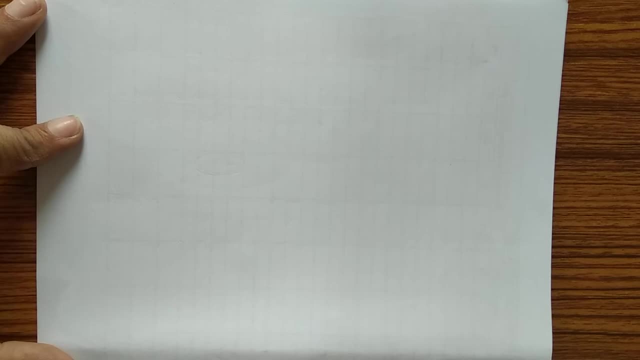 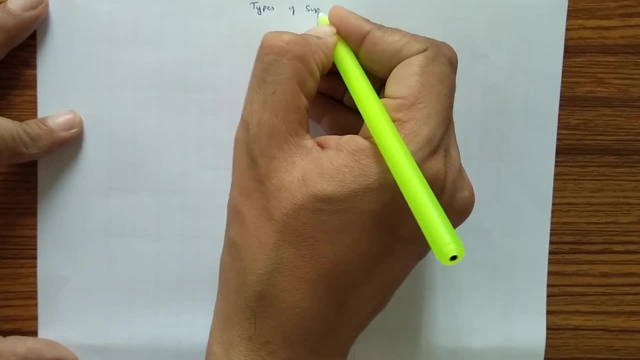 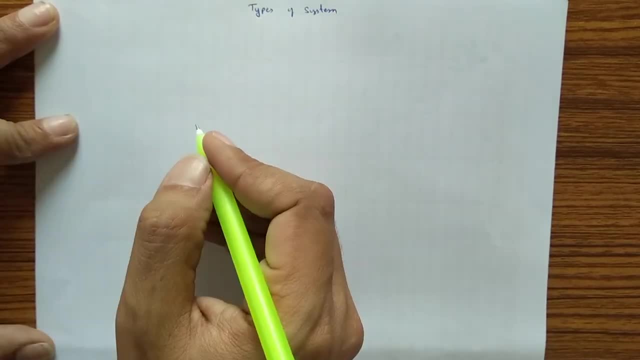 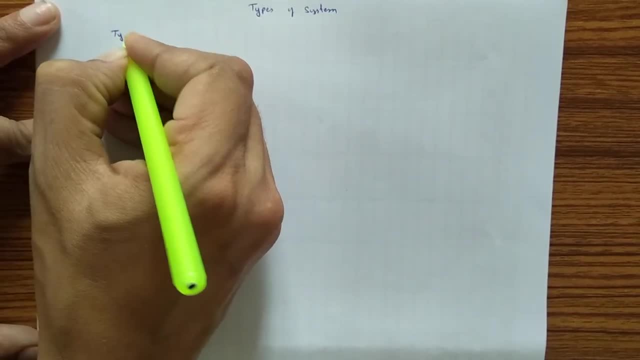 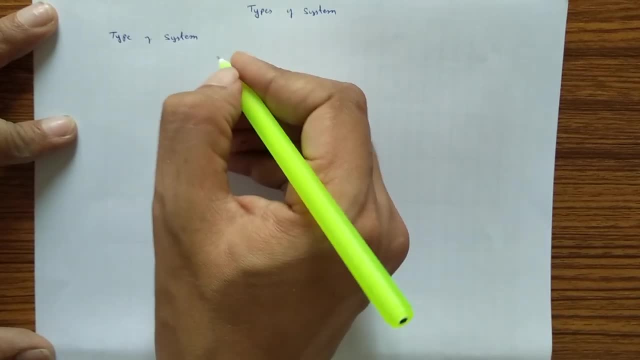 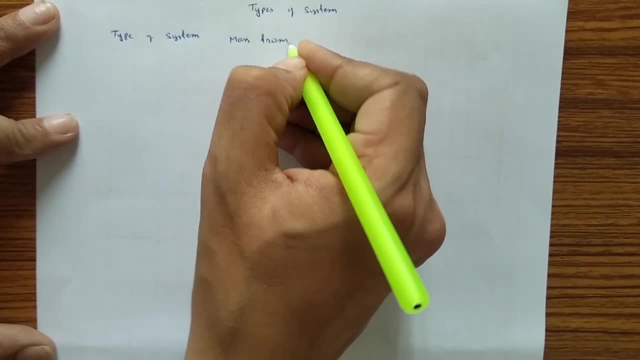 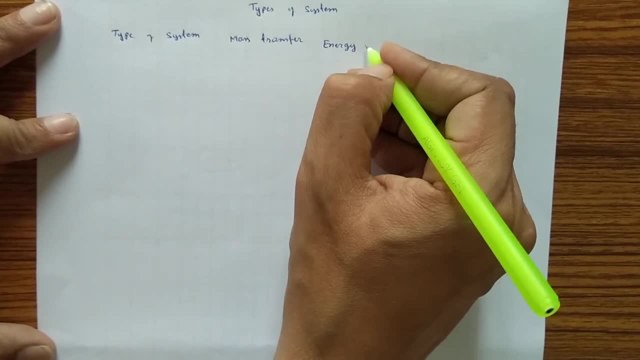 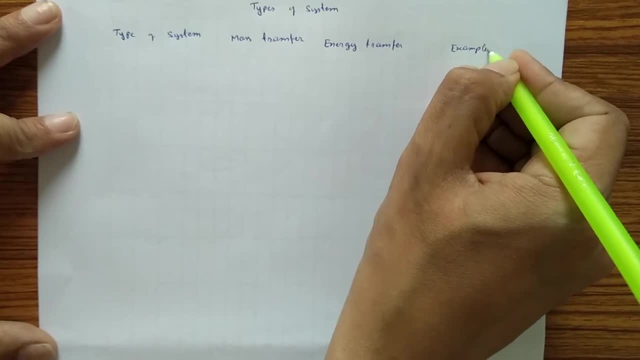 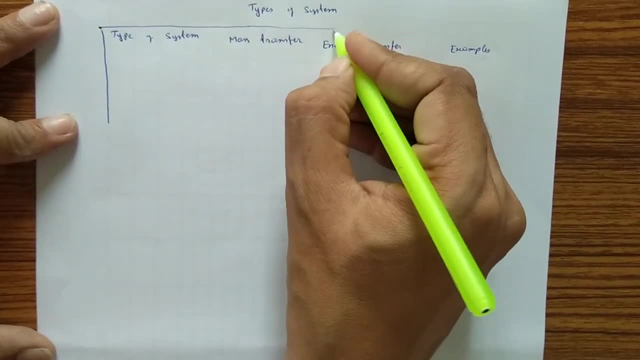 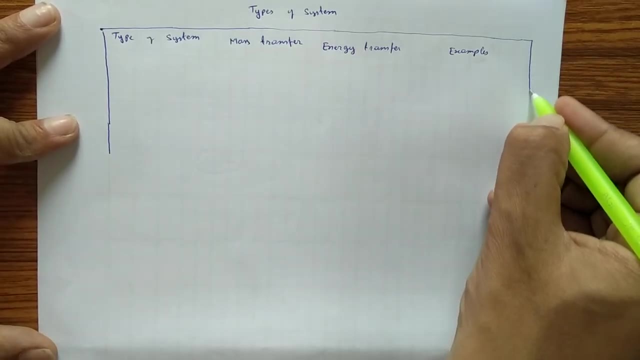 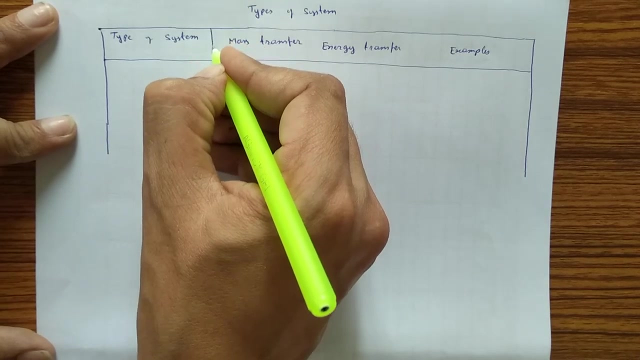 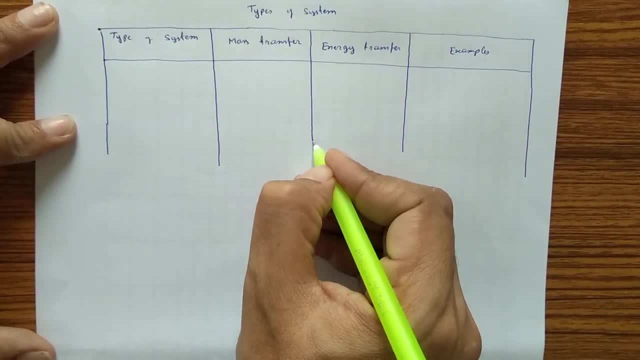 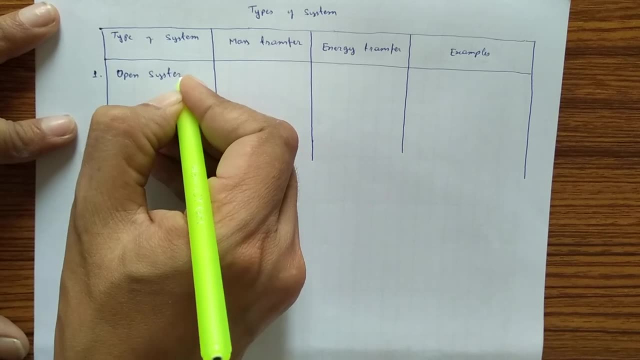 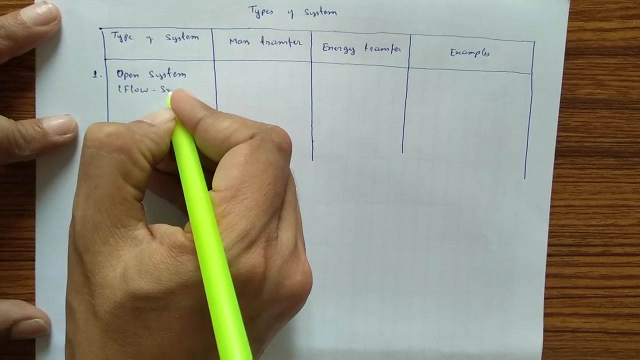 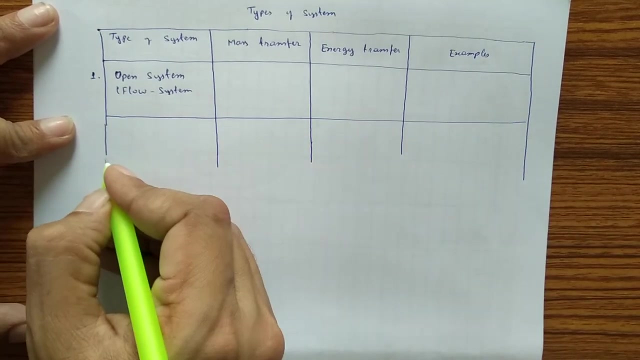 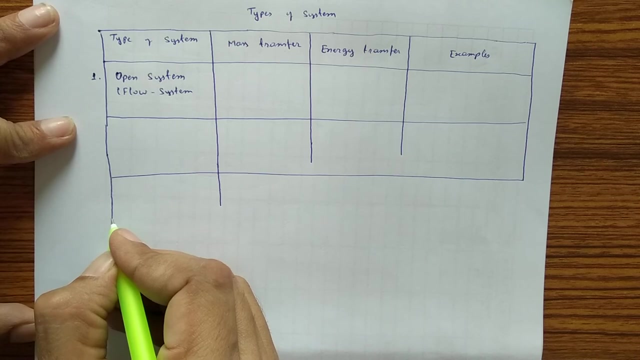 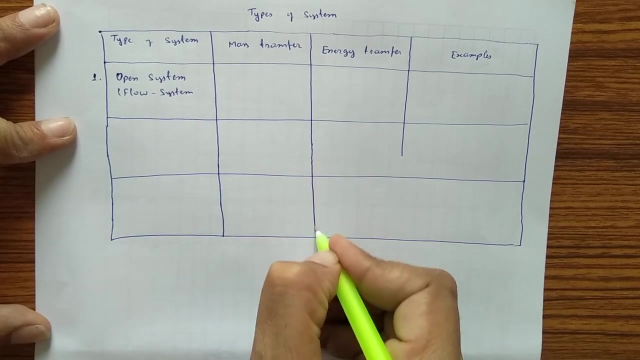 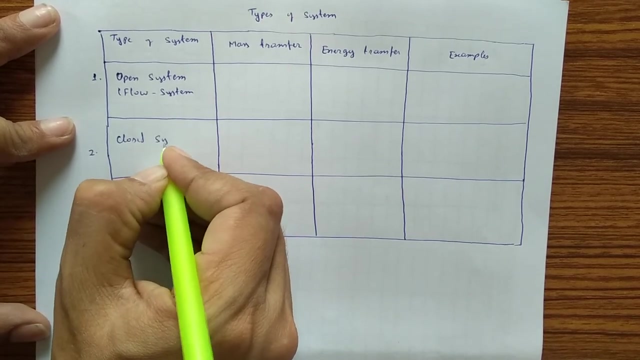 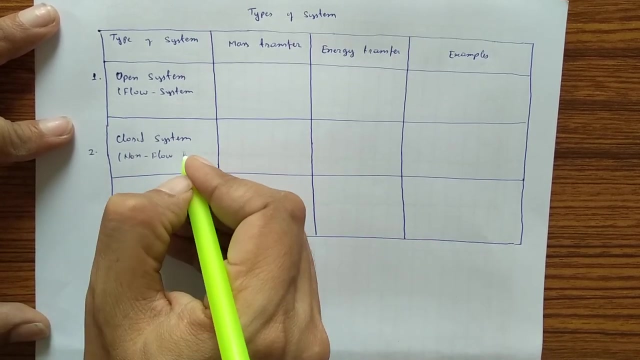 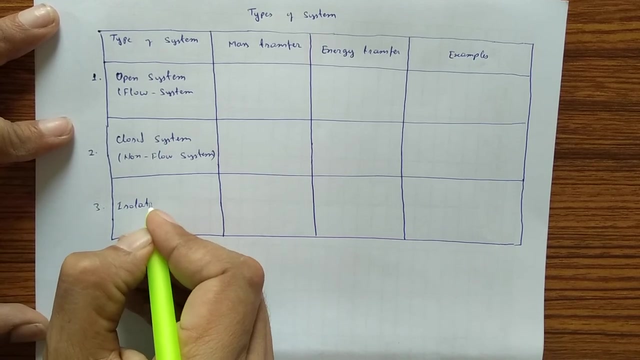 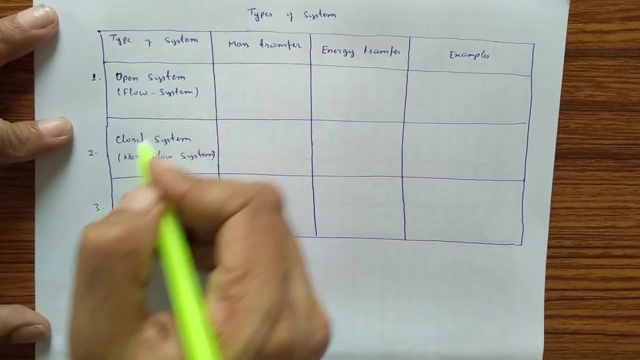 and examples. so if we see first, one is open system, it is also called flow system. the other is closed system, it is called non-flow system, and the third one is isolated system. the type of system are of open system, which is flow system, closed system, non-flow system, 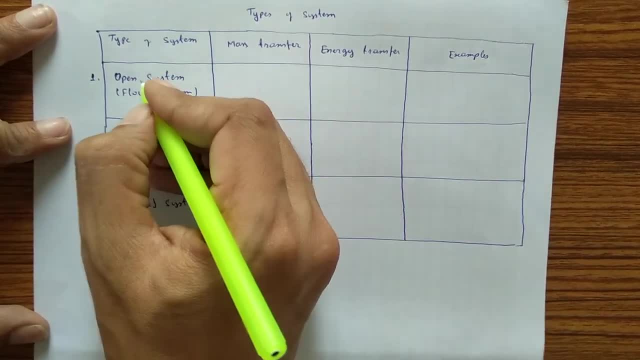 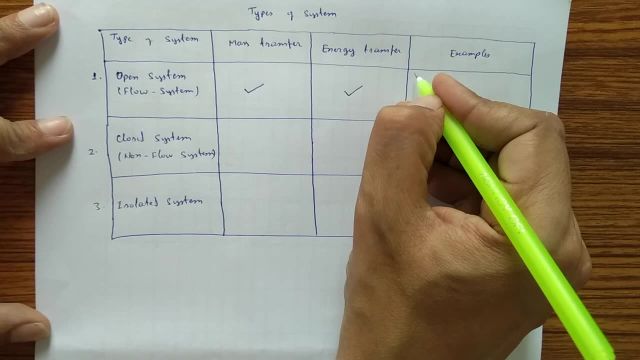 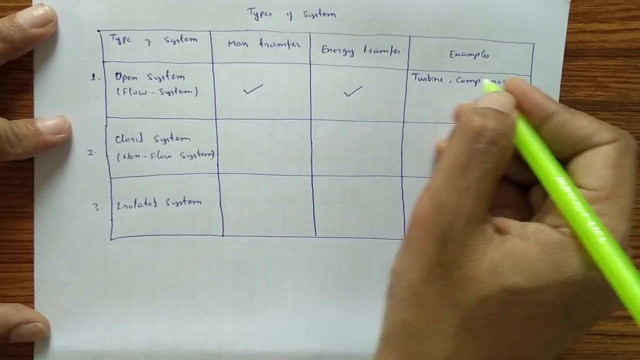 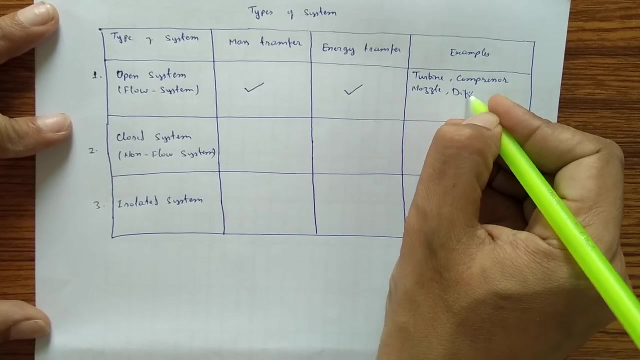 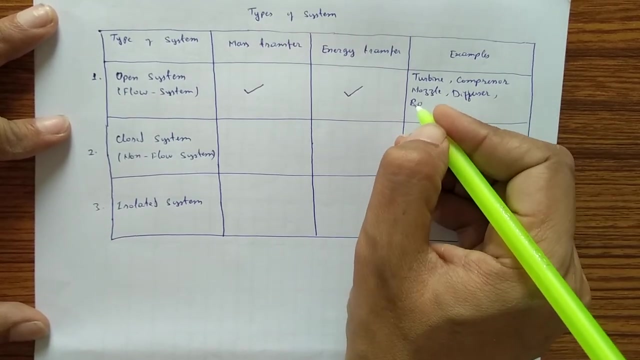 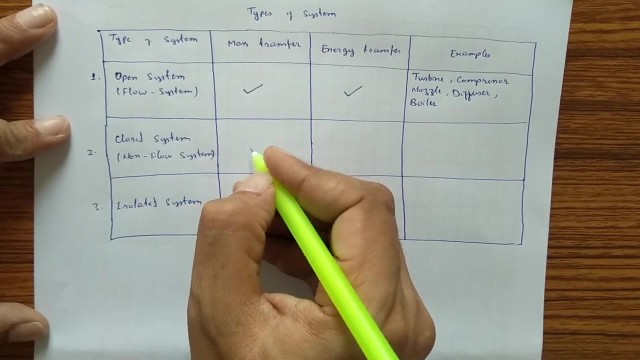 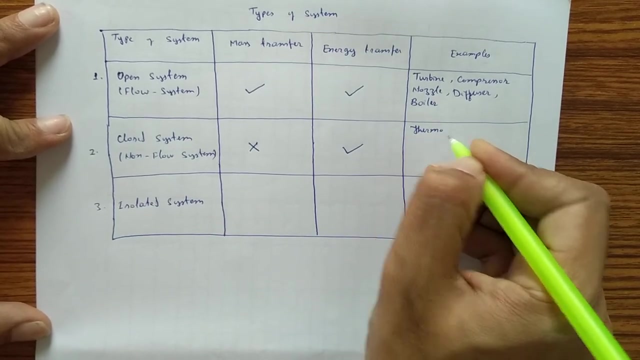 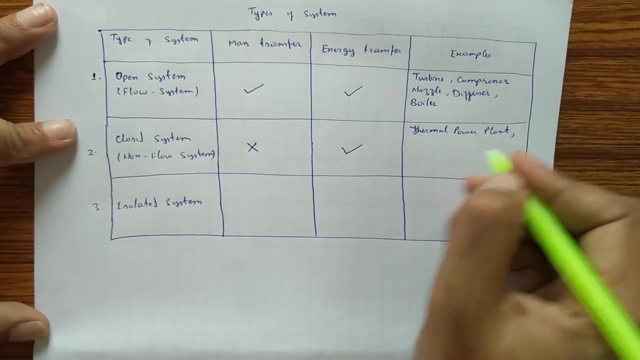 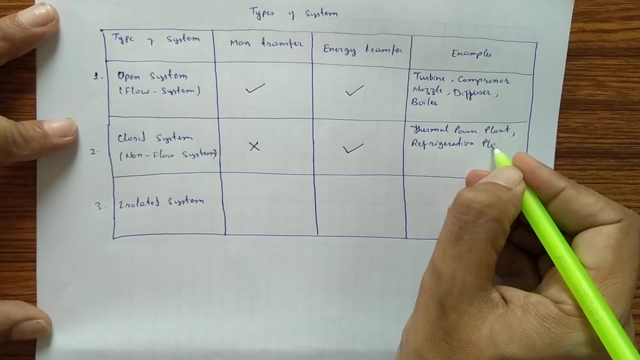 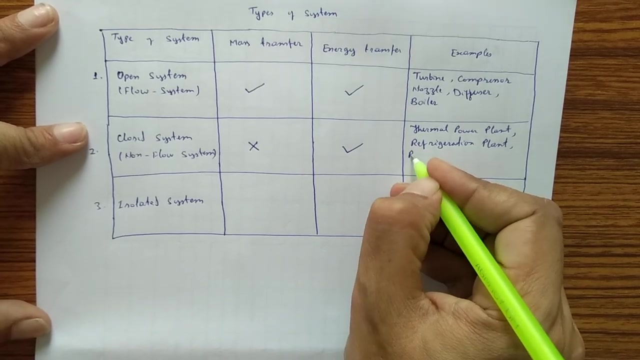 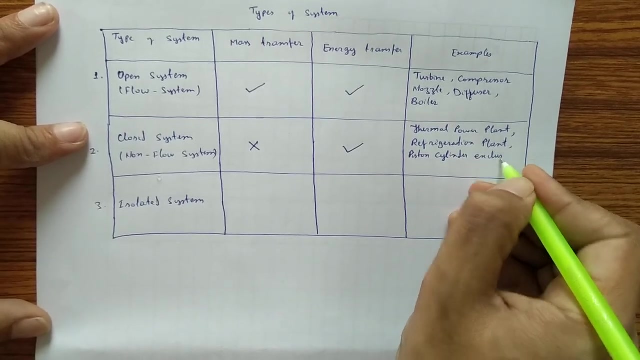 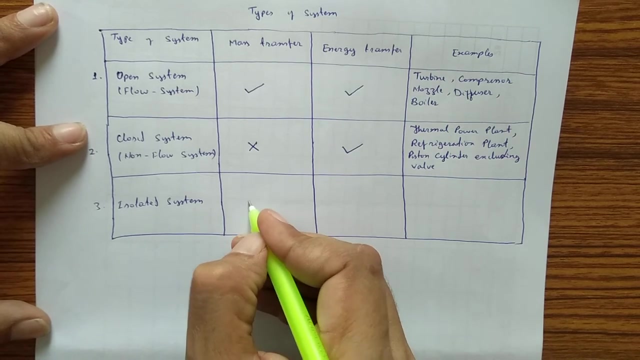 isolated system, but flow system. in flow systems, mass can transfer, energy can transfer. example: turbine, compressor, nozzle, Diffuser, Boilers, Close system. there is no mass transfer, only energy can transfer. example: thermal power plant, refrigeration plant, piston cylinder Including valve- Isolated system: there is neither mass transfer nor energy transfer. 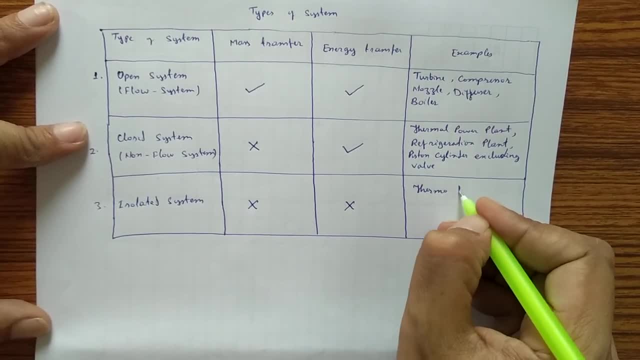 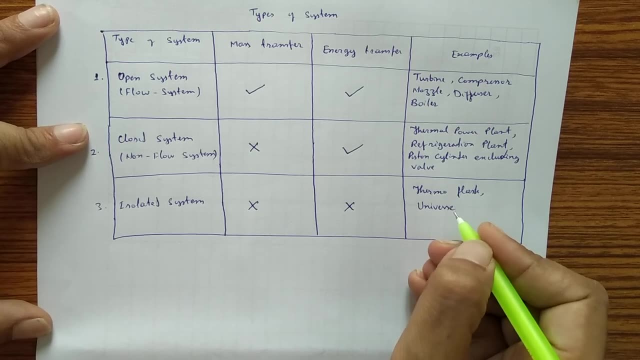 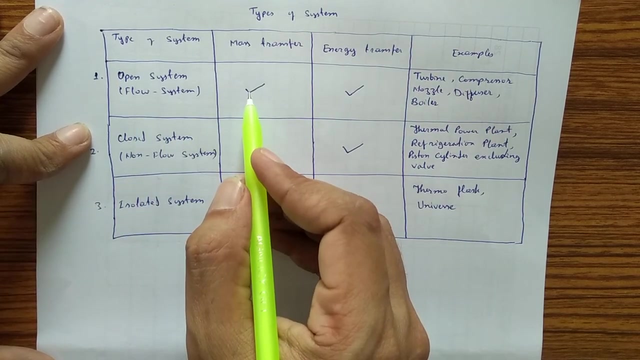 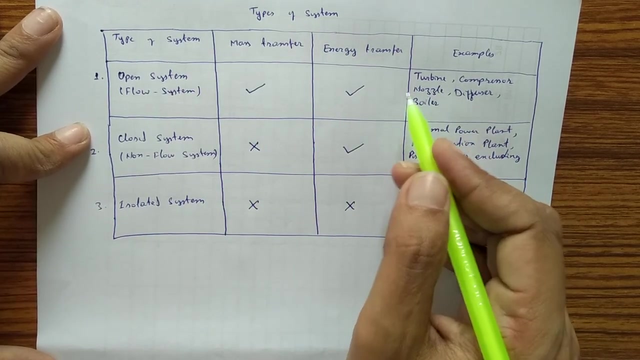 example thermo flask Universe. so type of system is open system, that is flow system. in this system mass can transfer, energy can transfer. that is both mass and energy, both can transfer. for example turbine: turbine: mass and energy, both transfer. is there compressor? 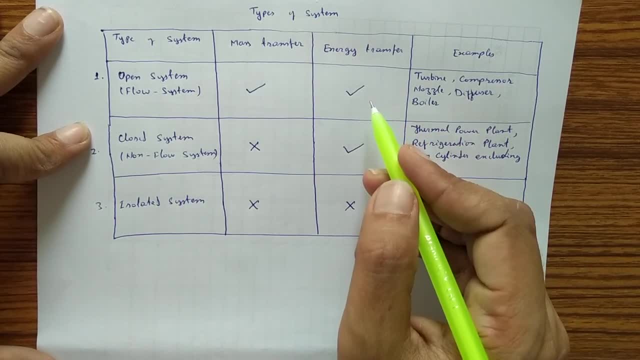 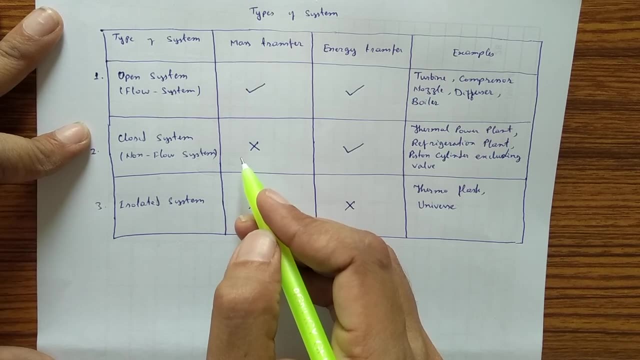 nozzle, diffuser, boiler, these all having mass and energy both transfer. other is close system, that is non flow system. in that system there is no mass transfer. mass cannot transfer in this system but energy can transfer. for example, thermal power plant, we get energy. 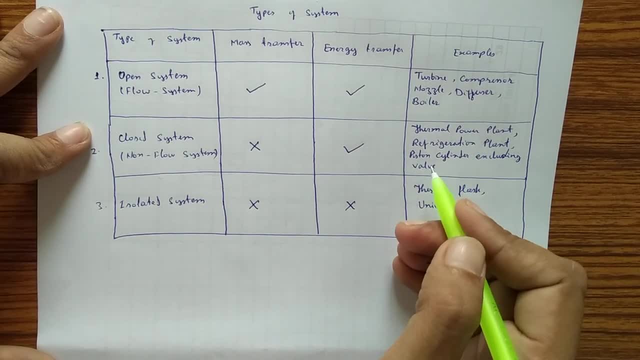 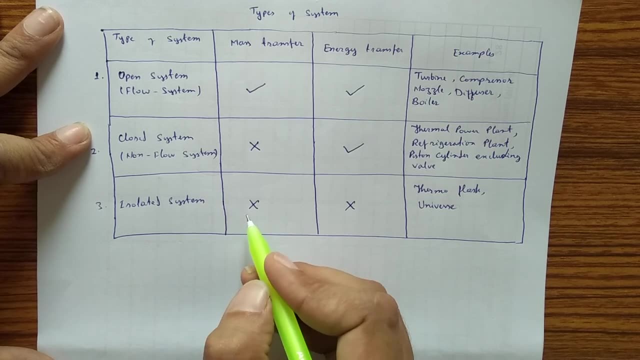 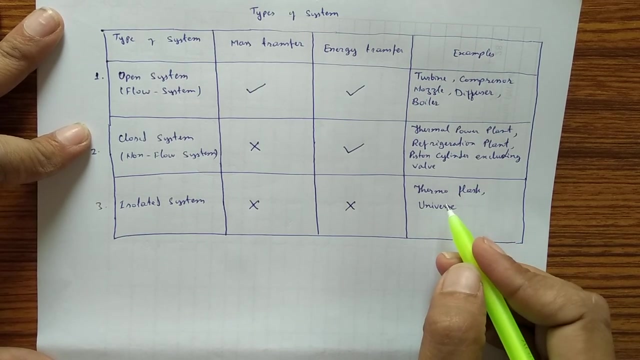 from thermal power plant, Refrigeration plant, Piston cylinder, Inclished piston cylinder, Temperature ceilingsschaft filter valve. So here also this is a星 system left hand side saving room. Voyage system- Here also it is left hand side saving well for the SA. 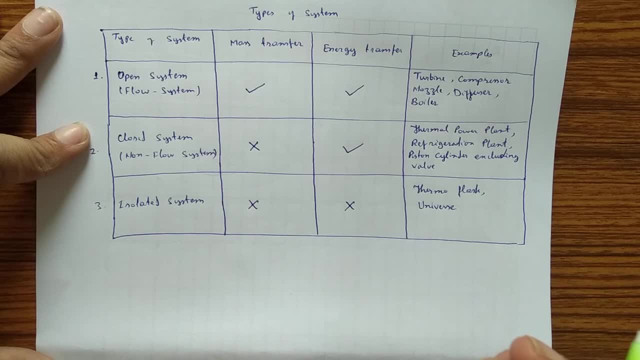 For thermo flask, there is no mass transfer nor energy can be applied to the system. unit using place is possible. for example, thermo flask. there is neither no mass transfer nor energy can be transferred. In case of this liquid in hot condition, it will get hot without any loss. because this: